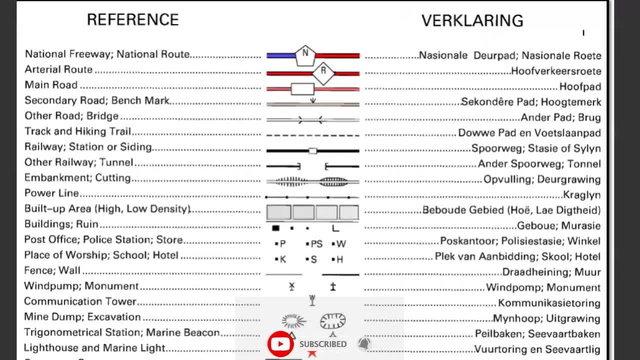 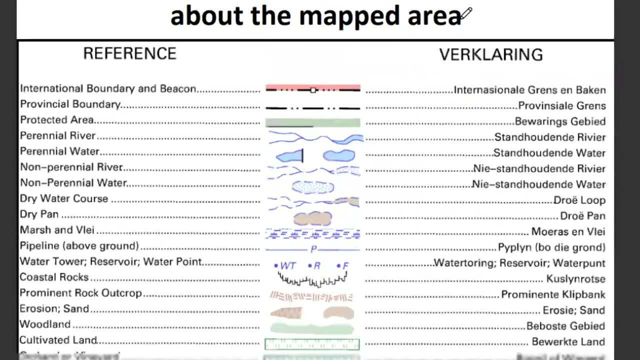 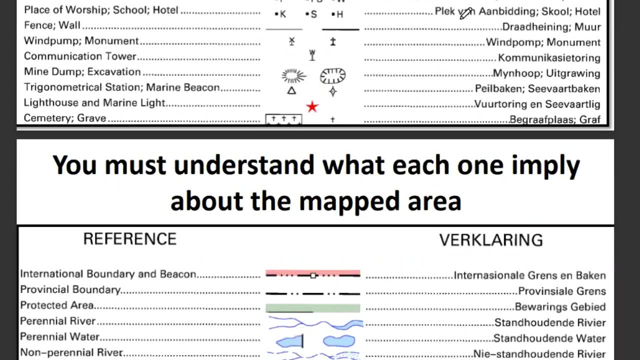 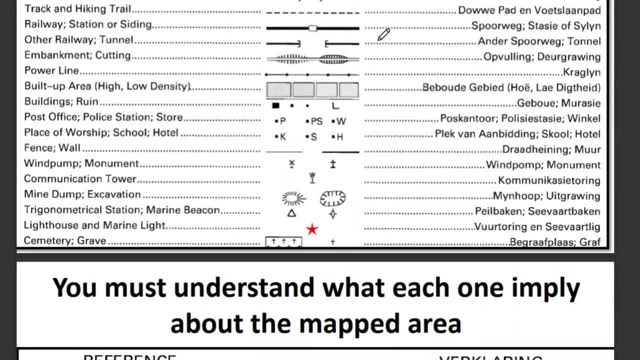 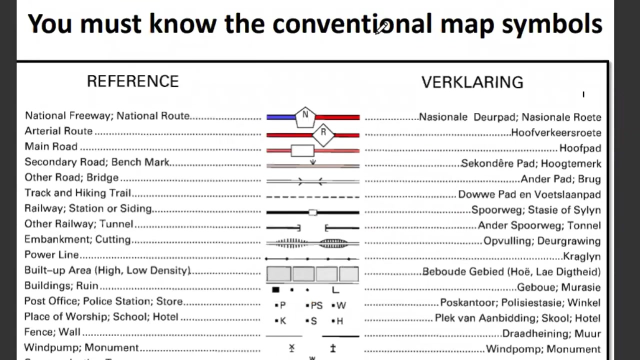 Hello, good day learners. Goodfrey's here to continue with the section that we left hanging, That is, the section for map work. Okay, And last time I was busy teaching or telling you regarding the interpretation of maps, calculations, application of geomorphology topic. 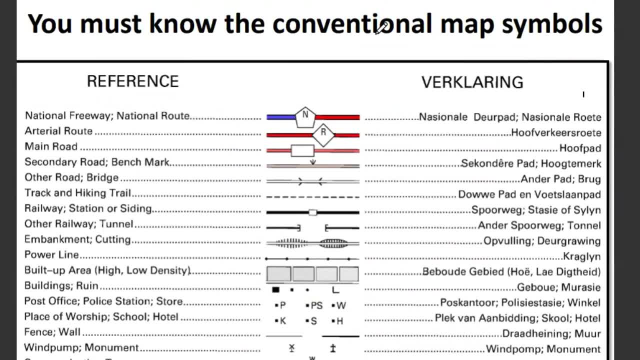 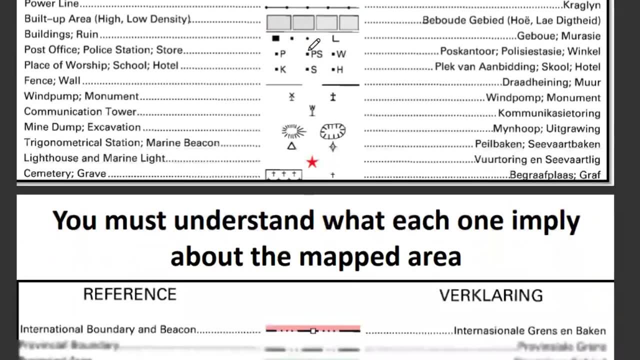 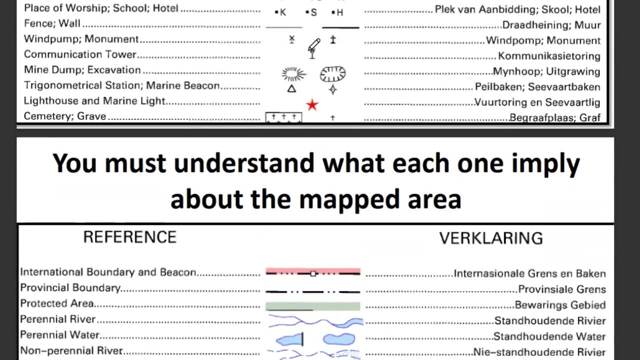 And now today I want to look at other related concepts to the application. Now, when you are given a map extract, please, learners, first understand that the map will be having this kind of things. It is what you call reference. Reference is a key. It's the key that you're using to try to interpret. 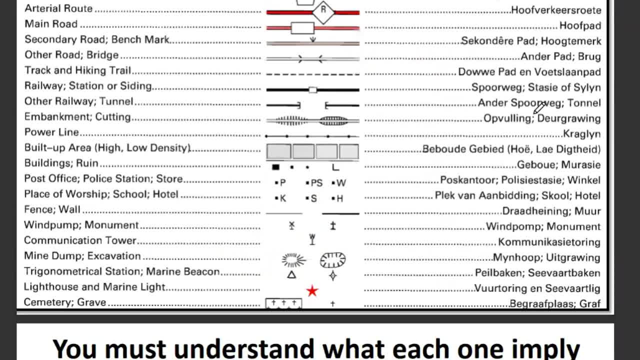 what you're doing And it's the key that you're using to try to interpret what is on the map. And if you look at it clearly, one side is Afrikaans, another side is English, So for those ones who are understanding Afrikaans, you can use the other side. 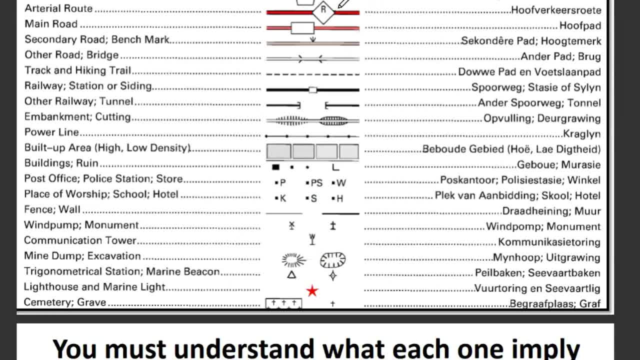 This side here. For those ones who are understanding English, you can use this side. But now I have realized that some learners are struggling to understand what the key or the reference tries to refer to. Please listen, learners. It is very important to. 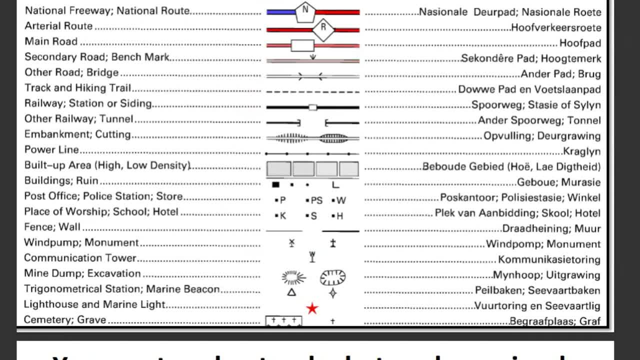 understand what the different symbols or convectional signs mean. A guessing point, A decimal point? We have got this, This part here. We have got, uh, this part here known as the National Road, And if you want to see what the National Road shows, National Road shows this. 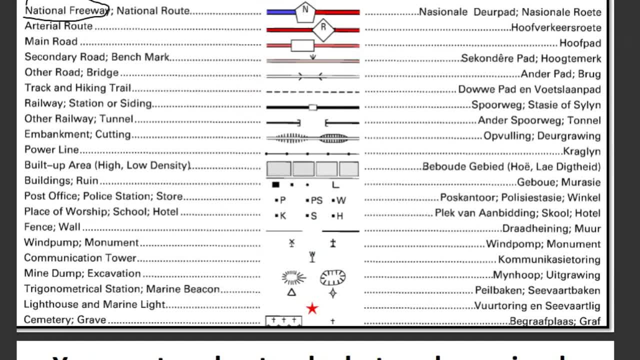 first part, which is blue in colour, This national route. It shows this other part, which is red in colour. So when you're interpreting you must know that this one, the first one, is for a first line, The second one is for a second line. We have the arterial route. 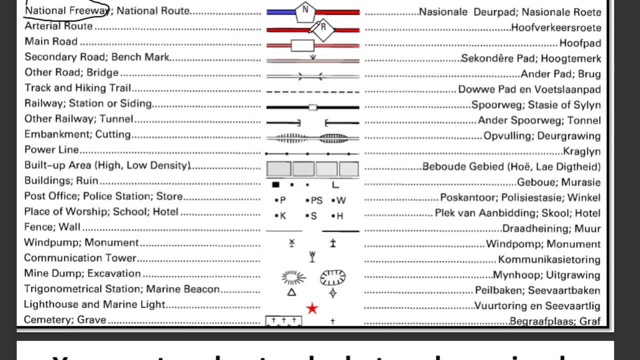 You can see the arterial route. there is one word, And if it's one word, you can see that it's completely one word. It's all red color with R in between, which means it's the arterial route, The main route. you can see it, same color. 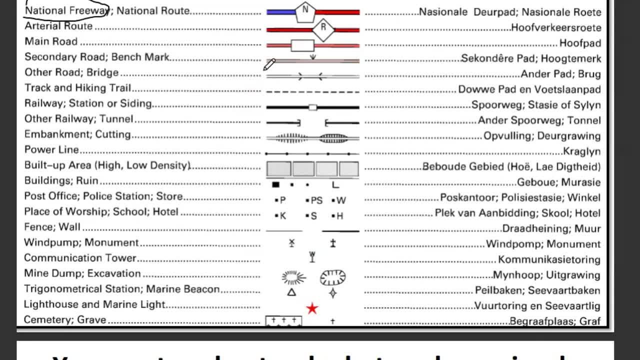 When you look at the second route I want you to see. The second route simply means this route that is having this kind of color, But now it is a benchmark. The benchmark is this symbol here that you see: Okay, other roads, this one, and the bridge is that sign that is just on the other roads? 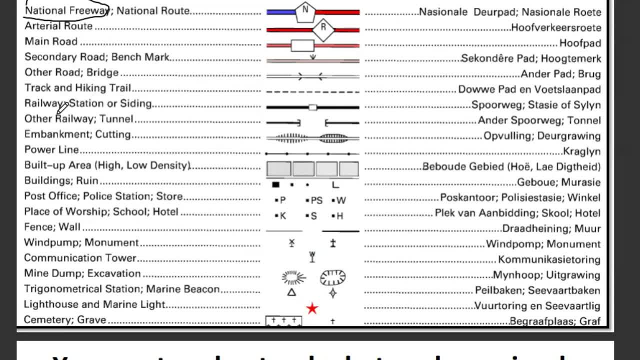 Tracking and trail. you can see track and hiking trail Railway station and the high railway station or siding. you can even see this black color here. So this symbol here, or this convection sign, is for a station Embarkment. you can see this is an embarkment here. 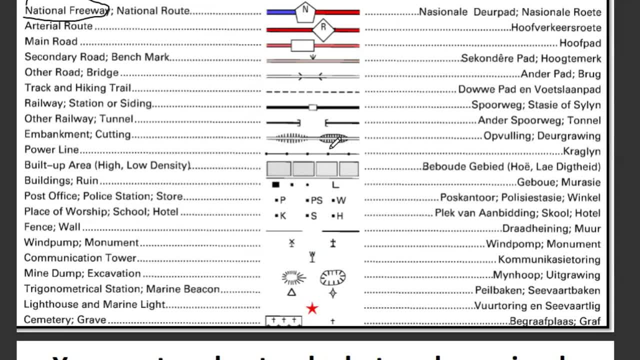 And then you have the cutting, which is this other side, Okay, The power line. In other words, you can be in position to interpret these symbols. I want you to look here Somewhere. here we have got a post office. 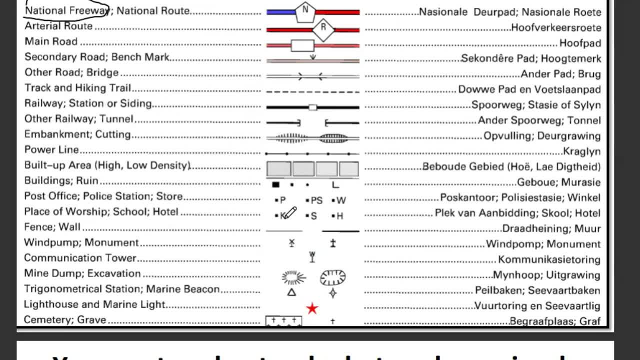 Okay, There is a police station and there is a store. Post office is P, Police station is P-S And store is W. That is its convection sign: A place of worship, school and hotel. This is a place of worship K. 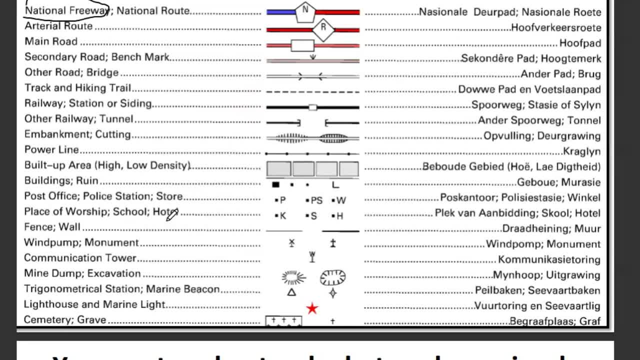 School is S And hotel is H. In other words, that is how you need to know to interpret The symbols. So the reference is basically assisting us to understand what is supposed to be on the map. So in this case, if there is anything that you do not understand and you just look at it, please don't just look at this reference as just given information just there. 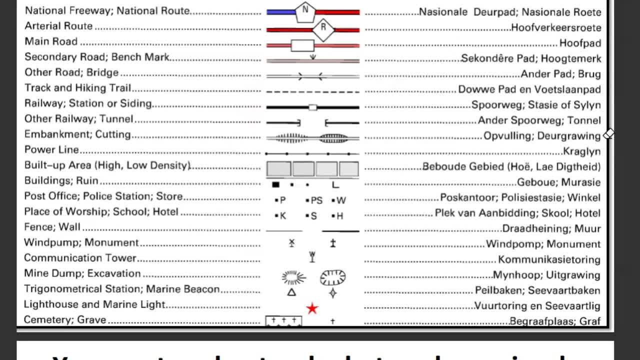 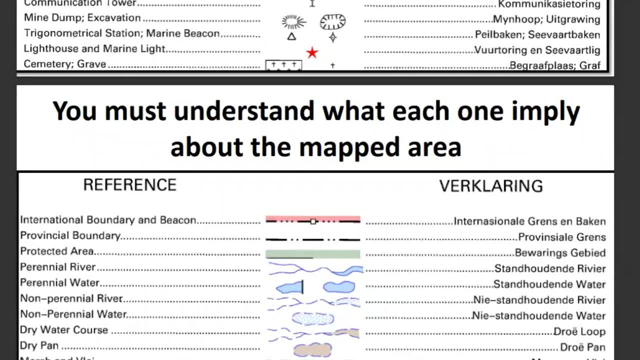 It's not irrelevant. It's very, very relevant for you to be in position to pass or to understand what the map means. So we must understand What each one imply about the mapped area. It's not only those symbols you see there. 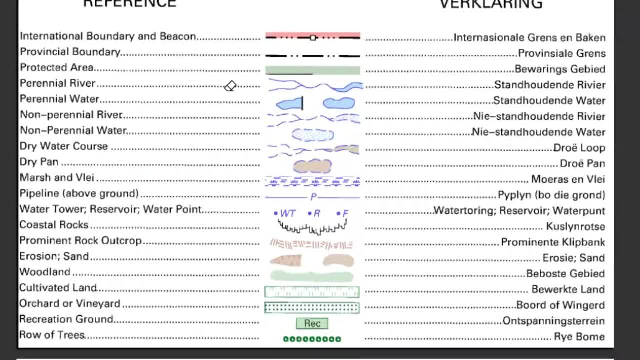 There are some other symbols. You can see these ones here. I know when you look at the kind of maps you have, in most cases you will find that some symbols are missing. But in case you have been doing with these other maps, you will see that a lot of symbols are existing. 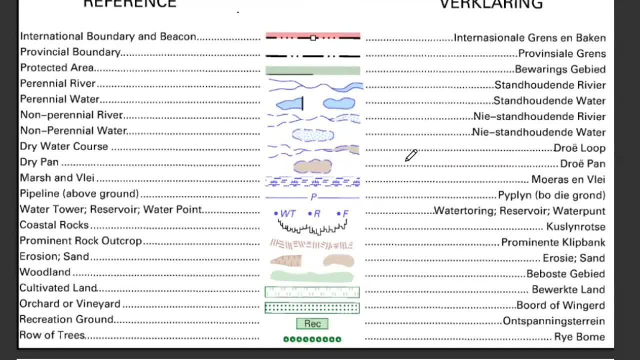 But now other symbols. You must be knowing them in your head such that you can be in a position to interpret them nicely. Take an example: The national boundary and the beacon. See that, The national boundary, this kind of line here, and then the beacon, that other kind of line. 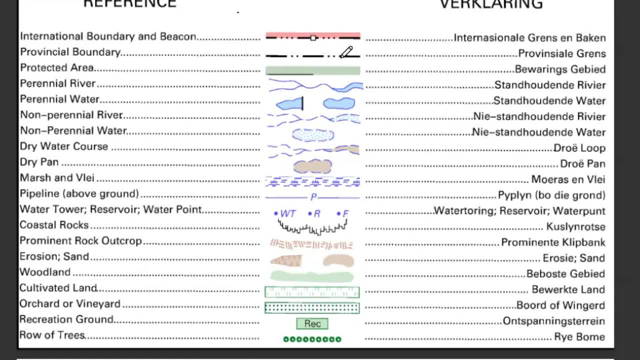 Then there is a provisional boundary. It looks like that. It's a bit different from this one. See, these are two dots, These are three dots. See that, So you don't take things for granted. Take everything very lever. 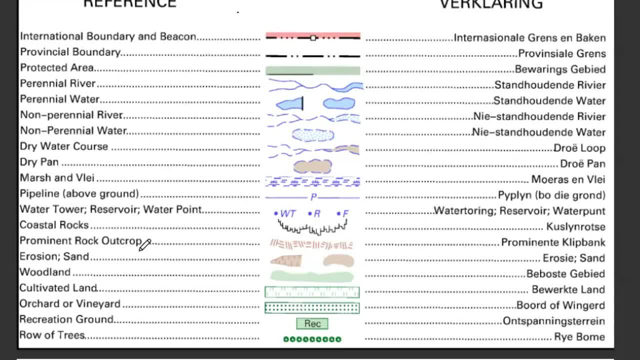 Take everything very important, And such things are very important. Take everything very important Such that you can be in a position to work with it. We have here a water tower, a reservoir and a water point, So this is a water tower. 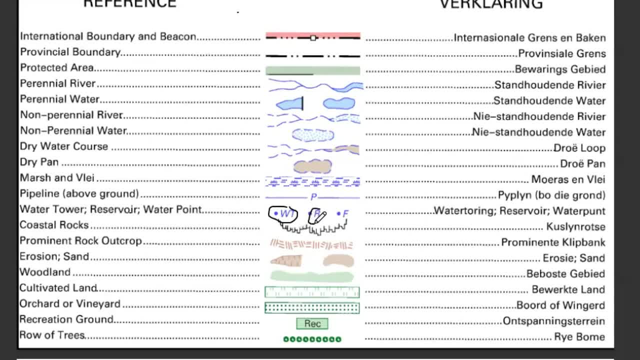 A reservoir- This is a reservoir here- And then a water point. The water point is aggregated with P- I mean F- Then we have a coastal rock. So this symbol is for a coastal rock, So on and so forth. So in other words, I wanted you to understand that in map work. 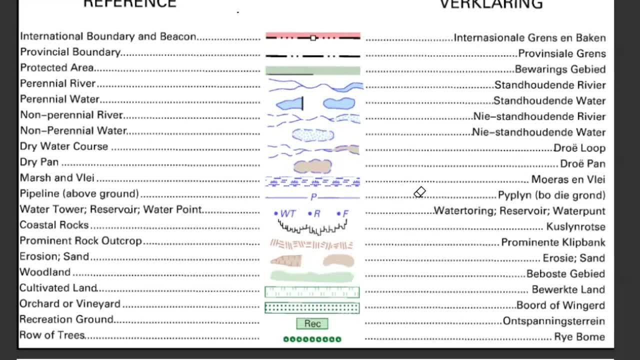 every symbol is important symbol. everything you see has got value, okay, so you must be in position to interpret. so, before you proceed with understanding both the geomorphology, the climatology, how settlement is applied, how economic geography is applied, please start by understanding what the difference 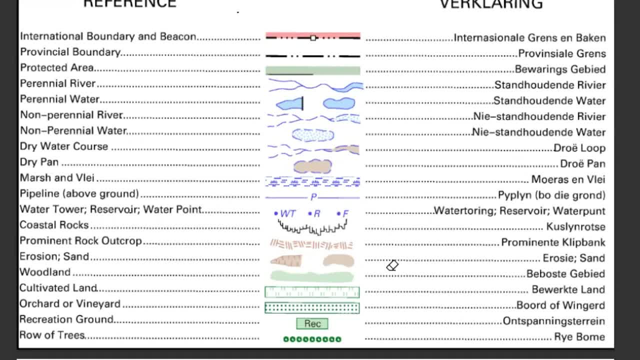 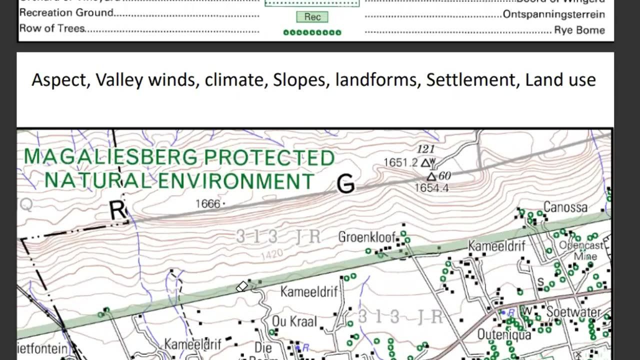 means on the mapped area, so that you can know that this is this, this one is this one, this one is this one, and that will assist us to be in position to interpret what we have on the map. okay, like i told you that it is interpretation, all right, learners, it is interpretation with. 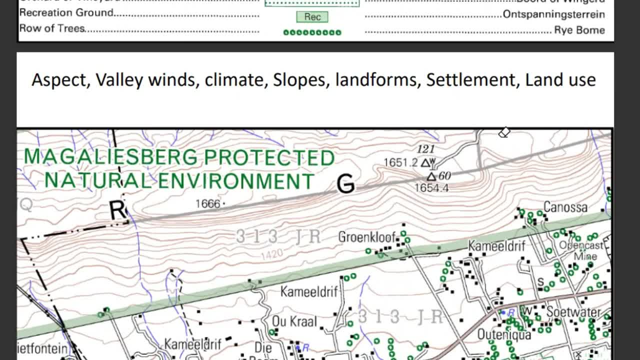 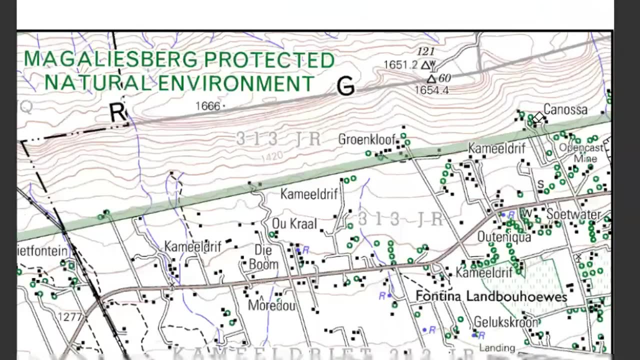 interpretation. we must make sure that we apply all the theory that we have learned so that it can be seen on the map. take an example: we have now looked at the aspect valley, winds, climbing slopes, landforms, settlements, land use and all that. so we must be in position to interpret all. 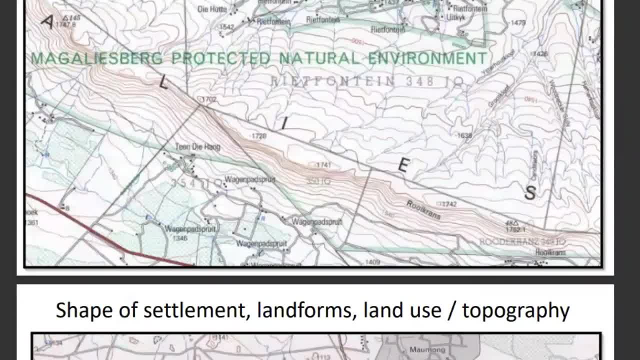 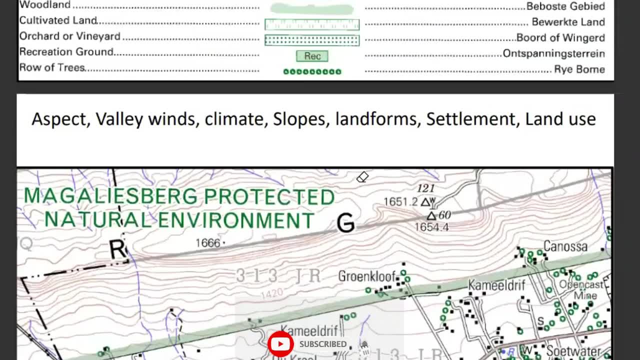 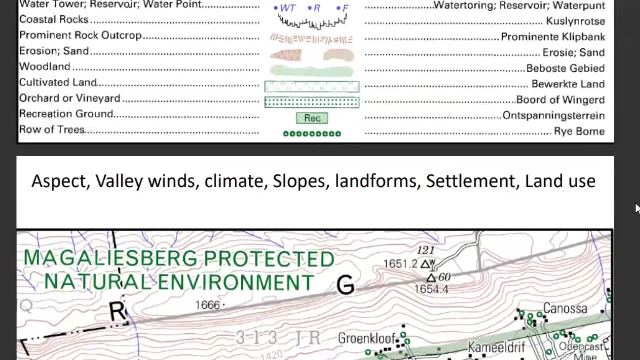 those aspects on the map. okay, so i want you to look at this. what do you see here? here you can see the issue of aspect valley, winds, climate- you can all apply it here- and settlement, by just mere looking at what each part is meaning. take an example. 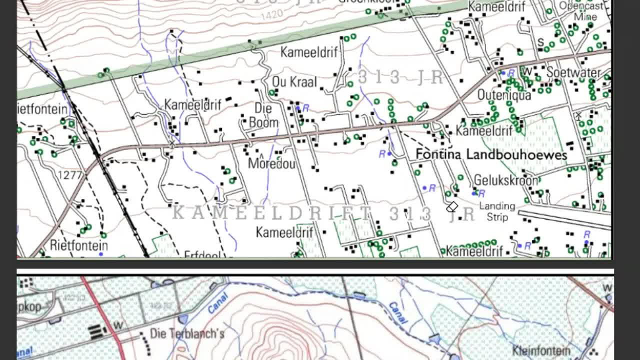 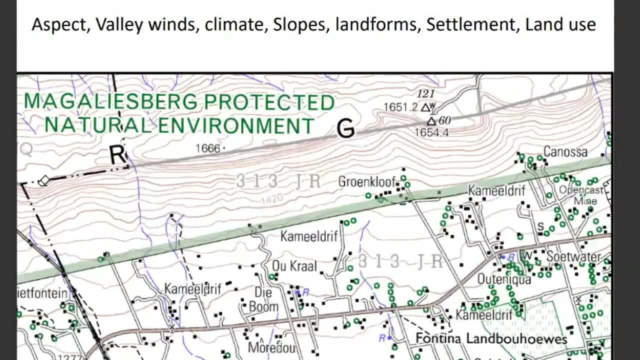 okay that when you look at this kind of map and when you check somewhere here, you can see the contour lines here depicting that this part here is steeper than these other areas, which is basically a slope, a steeper slope here compared to what is happening this other side. okay then, here is a protected area, natural protected environment that. 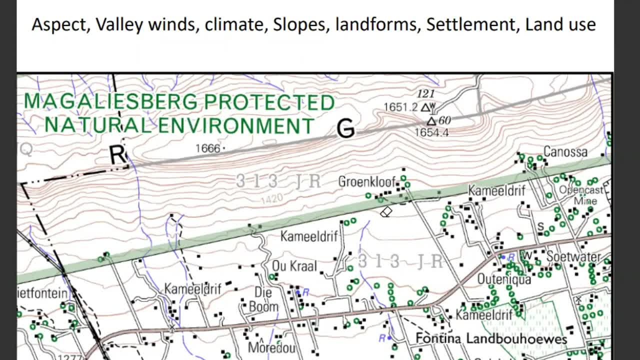 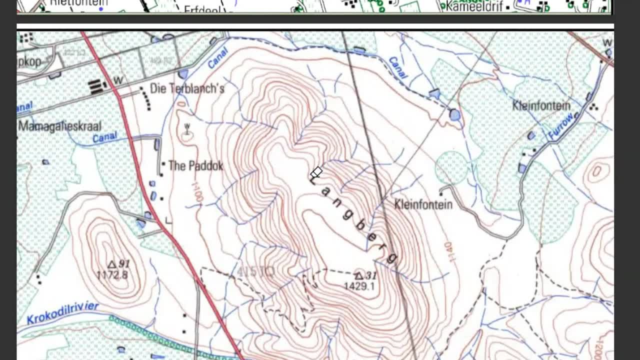 can be a game park, a game reserve and so on and so forth. so you must be pushing to interpret that. when you look at this one, what do we see in terms of drainage? you can see that this is a high-lying area, so these rivers are all draining outwards, which forms a kind of a pattern drainage in. 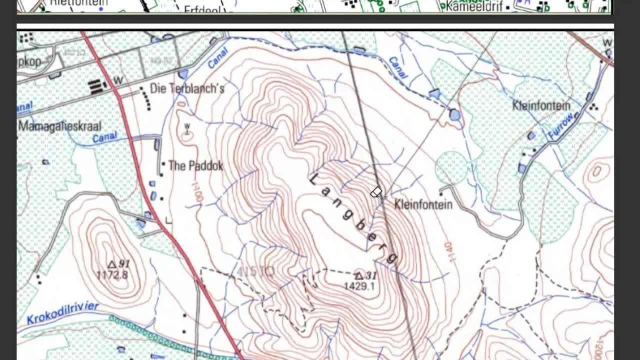 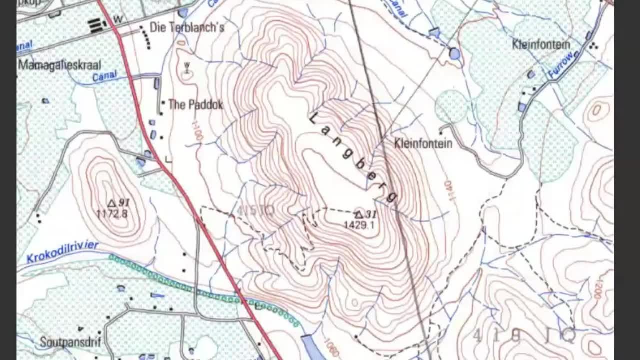 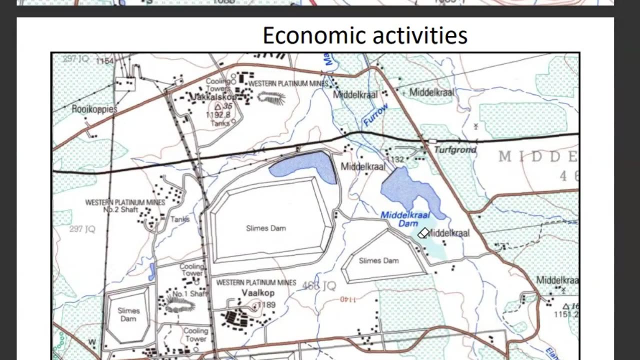 in geomorphology that we call the enderitic drainage pattern, and when you check somewhere outwards here it's lower than what is happening here. okay, now you can see this part here. i want us to be in position to interpret the economic activities. what do we see when you see this? this? 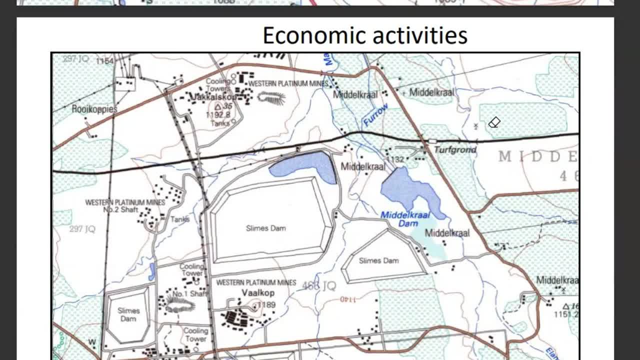 is showing the cultivated land. okay, and if we talk about the cultivated land, what do you expect? expect activities like agriculture, you expect activities like farming and so on that is likely to take place in that area. and to make it uh, to make it easy, easy to understand, you can easily interpret that this. 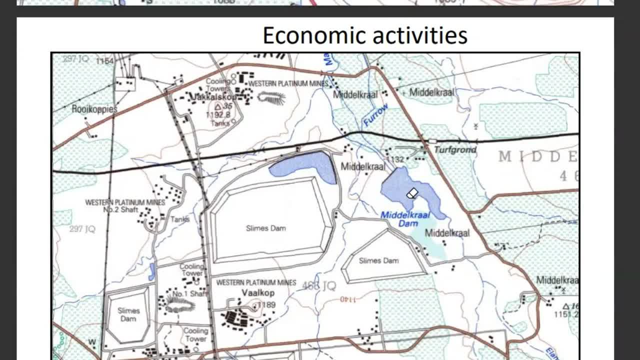 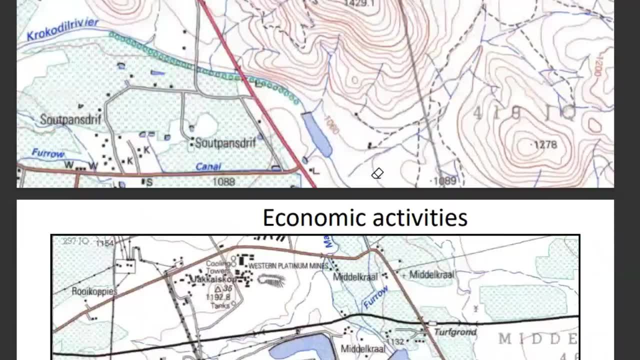 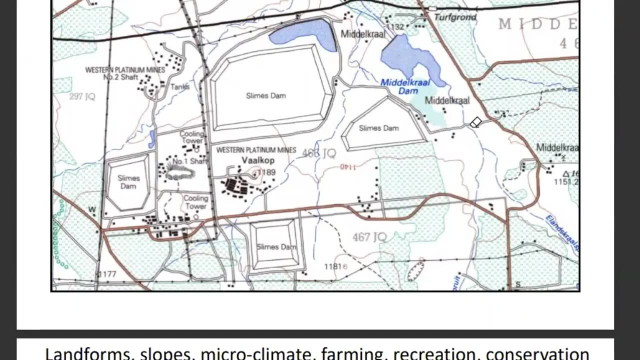 um, this cultivated land is basically located close to the dams, near the rivers and the furrows, meaning that they can easily have access from the dams to these farms and they use it while practicing agriculture. okay, besides that, there are some other activities that we can look at here. 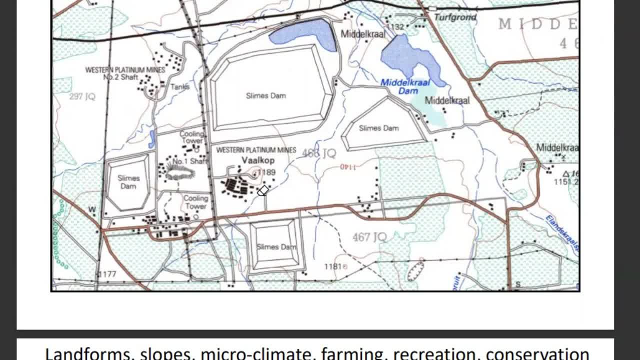 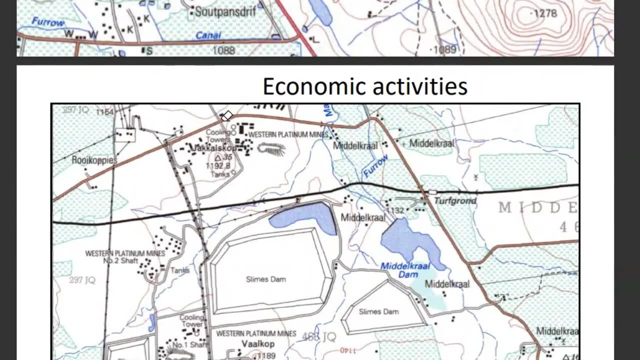 that we can think of. take an example: if you see here this is an excavation, okay, that means there's some kind of mining taking place. in that case, okay, then you can also look at this place where this place has got mining being practiced. take an example: we have what you call the western latin um. 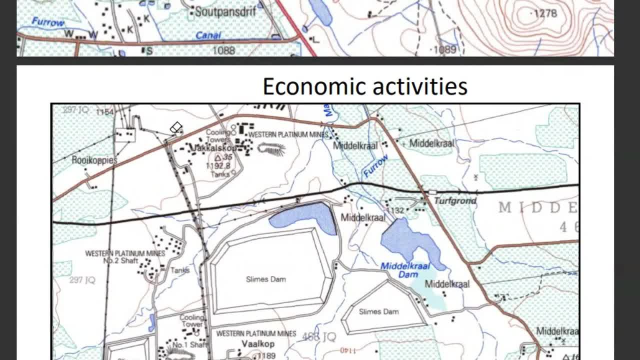 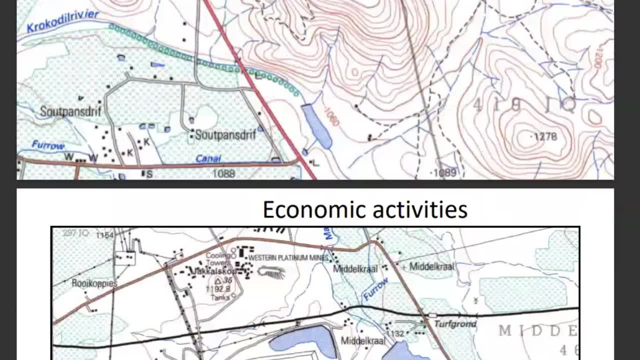 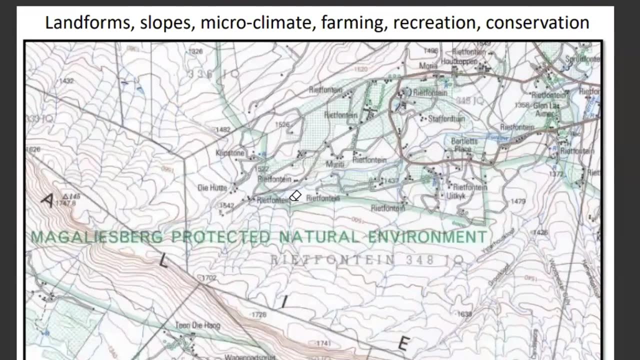 okay, western platinum mines, meaning that there is mining taking place in this area. this one can help us to interpret the economic activities that are taking place in this locality. okay, now we go ahead and look at the aspects. all these ones are applications. are applications or interpretation of? 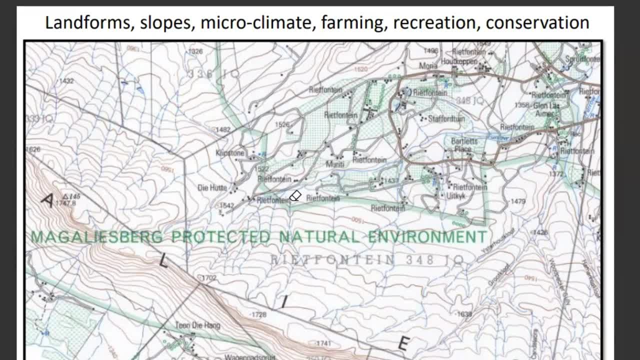 theory or map work with the different topics that we look at in geography. so, like i told you, that all aspects you look at are applicable: landforms, microplanning, farming, recreation, conservation and also and so forth. so when you check here, what do we mean by conservation? this is the 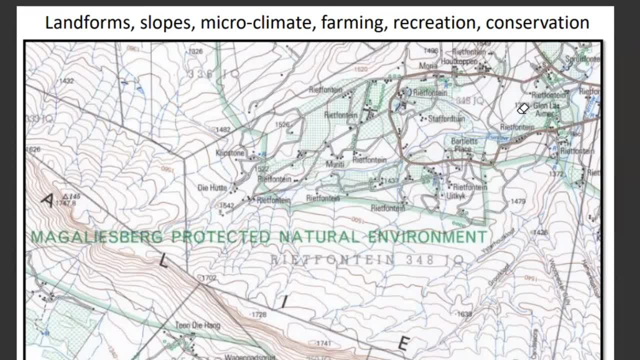 basically the using of the protection of the environment or preserving the environment for future use. when you take this area here, uh, my heart is back. protected natural environment- so my heart is back. protected natural environment is basically a conserved area, meaning that conserved conservation is taking place here. okay, when you see the cultivated land, what does that mean? 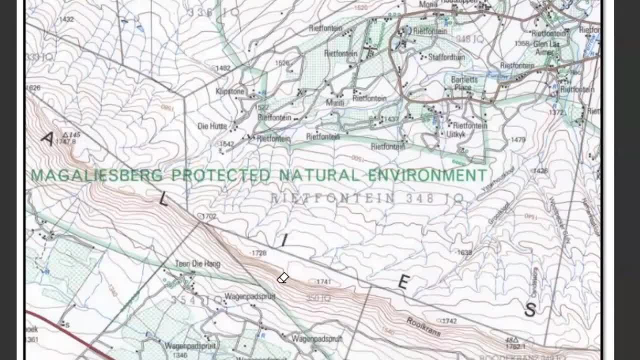 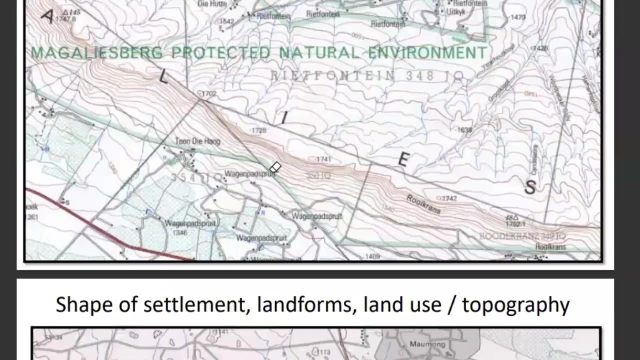 maybe there is farming taking place here, and when you see that this is a bit, a little bit steeper, what do we look at? we can think of, uh, the slope aspects. okay, we can also think of a microclimate that the climate that is affecting, affecting very small areas. so, in other words, all those 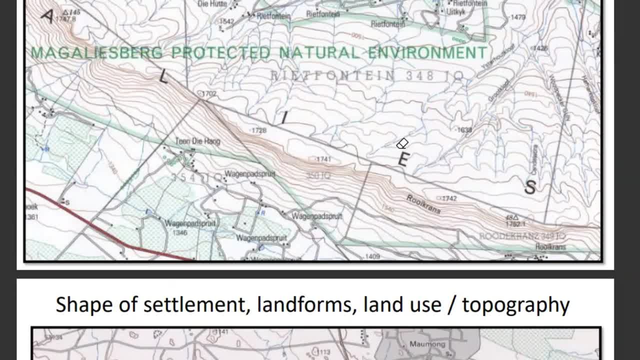 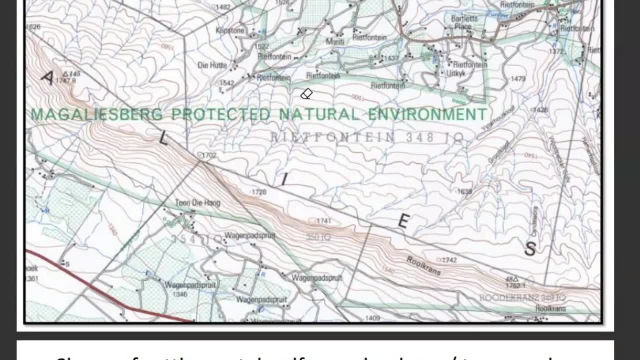 ones are trying to assist us understand the interpretation of maps using the different topics. okay, so learners understand that any time, any day, when you're writing your geographic papers, you're going to find out that those topics are going to come your way. you must be in position. 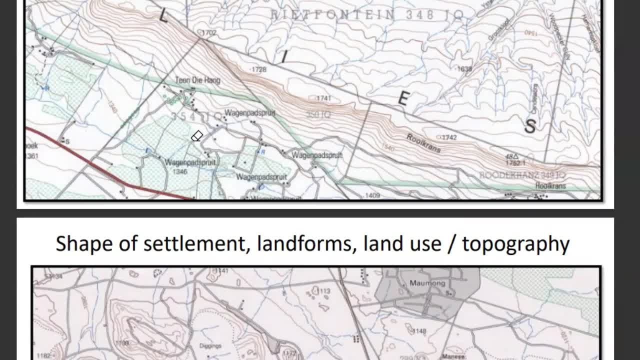 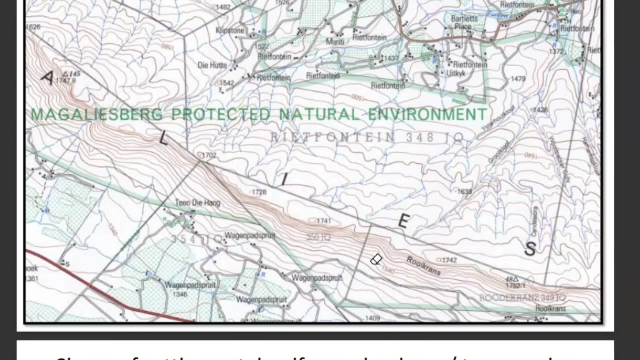 to apply what you have looked at in theory. it is going to be very difficult for you to understand the concepts when you have not applied the theory or when you lack knowledge in the theory. take an example: when you look at this slope aspect and you check this side, there is a lot of green. 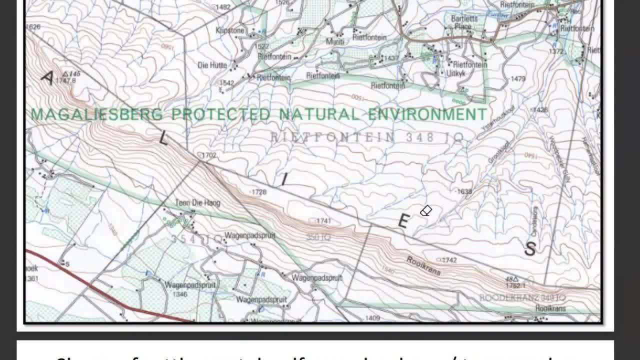 compared to what is happening. this other side, remember, when you talk about slope aspect, slope aspect you look at to uh, where the sun is facing in nation, where, where the slope is facing in relation to the sun, meaning that on the shadow zone, we said that that place is cooler, okay, so if you're in the southern hemisphere, the 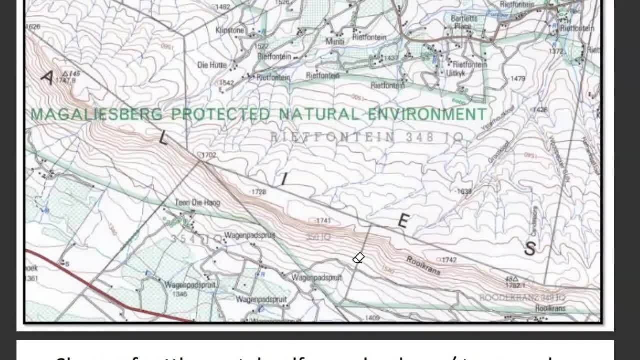 south-facing slope is much more cooler than the north-facing slope. what is? what does that mean? the south-facing slope can easily favor activities more like um, you can easily favor activities like the growing of forests because it's cool. remember, trees need a cool environment and when you check this other side, there's a lot of green this other side and there's 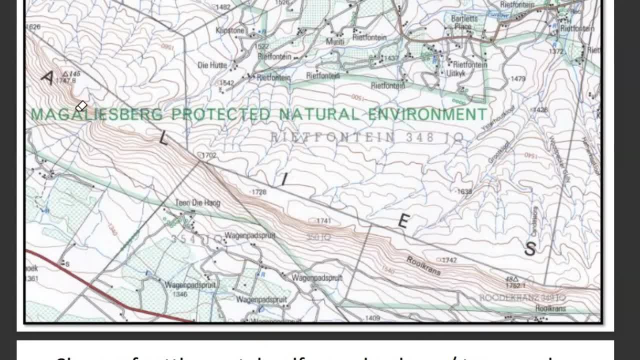 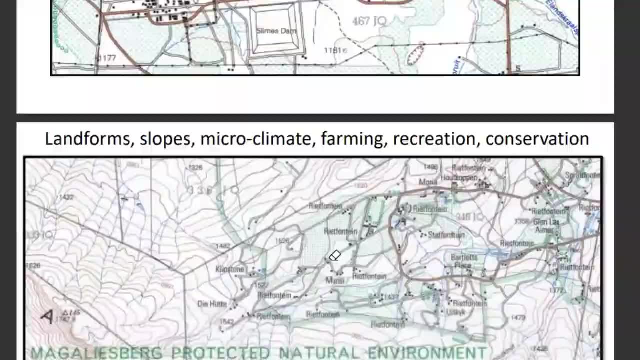 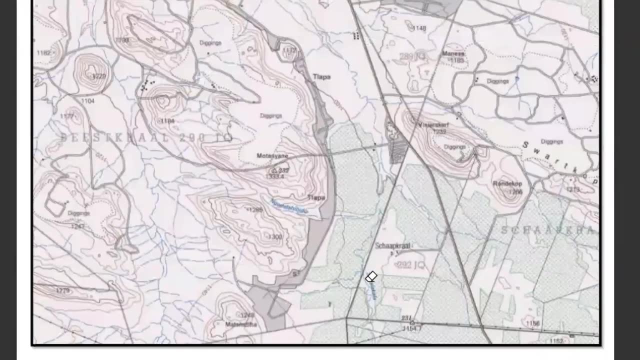 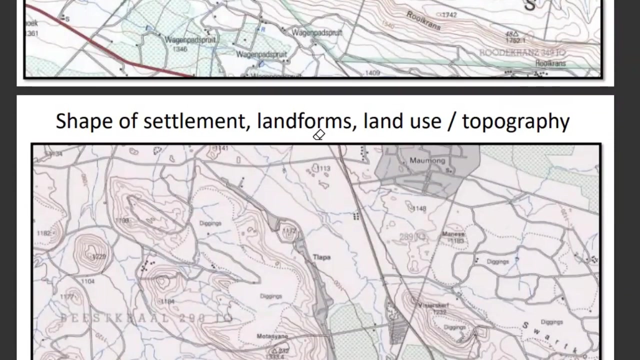 a lot of cultivated land this other side compared to what is happening on the on this other side. so i want you to be in position to apply. that is application. okay, be in a position to apply all right now. um other topics, both settlement- here we have what you call the shapes of settlement landforms, land use. 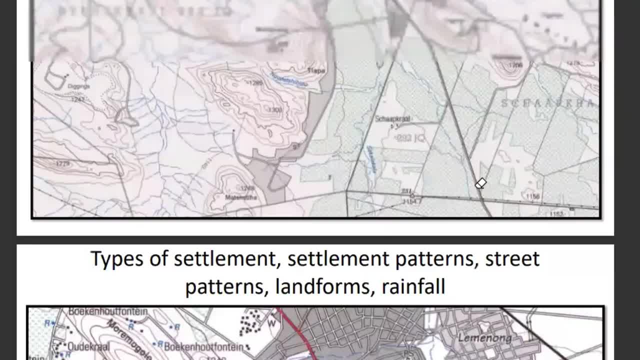 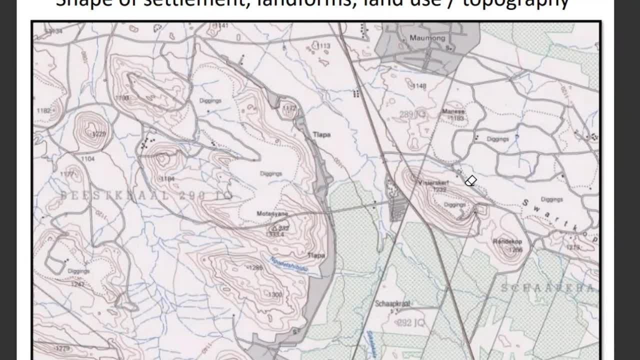 and topography. when you check around here on the maps, what do we see? we talk about the shapes of settlement. how many shapes do we have? we have a lot. we've got a lot of shapes, for example, the linear shape. okay, that is when the settlement is along a line. a line like what? like a road? 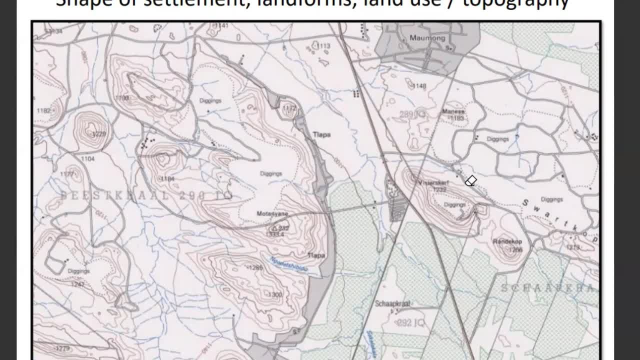 a line like what, like a railway line, a line like what like a river. so in this case, if you see a road like this and there are settlements along the road, which ship which ship is more likely to be formed? if it's along a line of a road, okay, the line feature that would be, there will be a road. 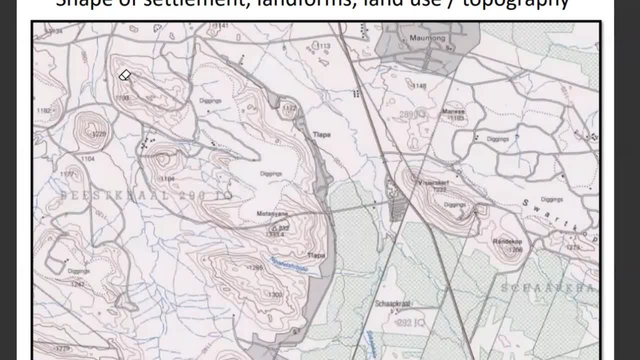 and if you see this road, that means you will know that the kind of settlement shape is a linear settlement that is taken place. okay, so besides linear, we have got what to call the star shape. beside the star we have got another shape like that is a circular shape. that is, for example, when the settlement is 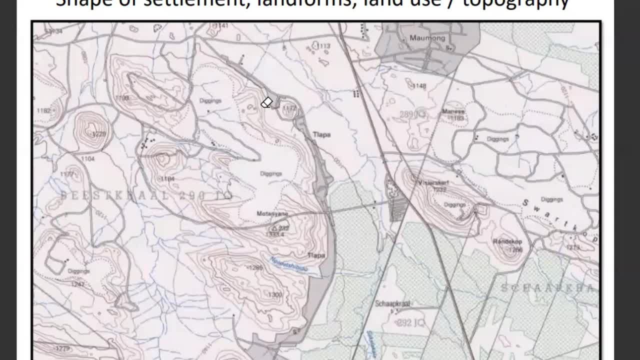 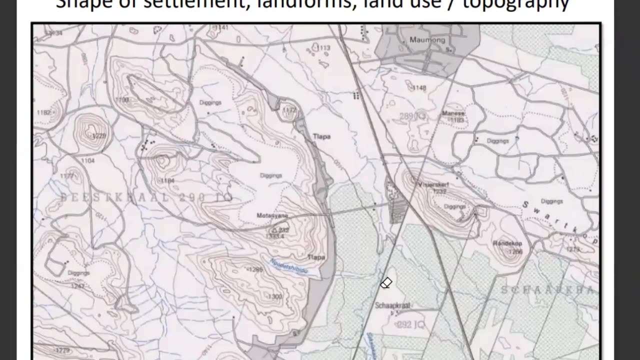 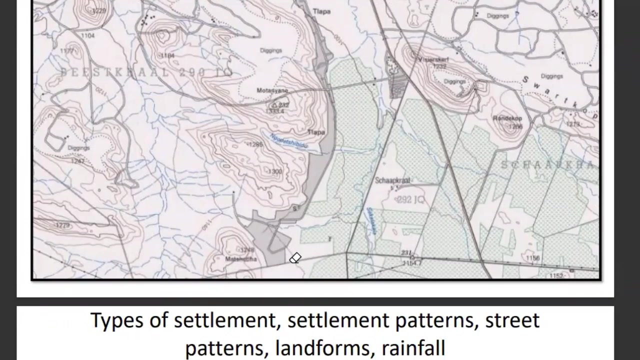 around, um, um, the circular features like mountain, like lakes, and i understand we have also what you call the semi-circular shape. for example, at the coast, at the coast, oceanside, you'll find that kind of settlement okay. so if they ask about the settlement pattern, what do you expect? settlement pattern will look at the layout of settlements. 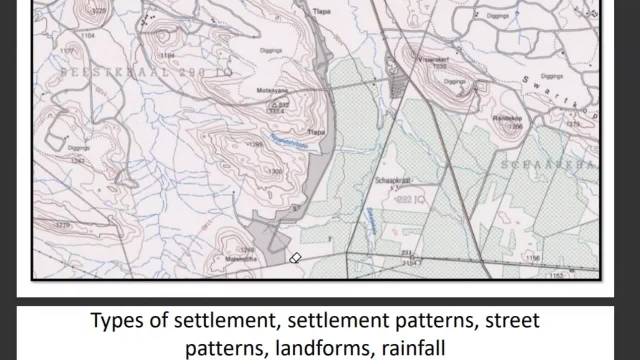 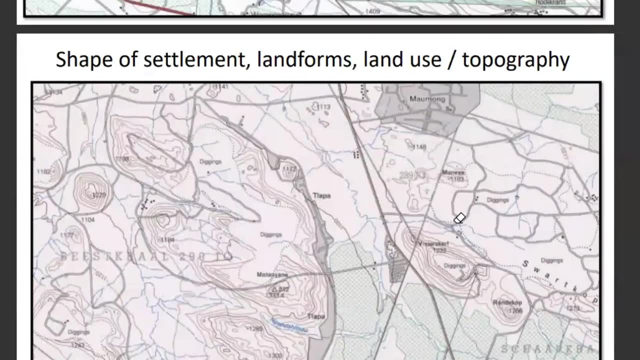 in an area and you find out that it's either nucleated pattern or sparsed. okay, nucleated or sparse, if it's nucleated simply means when the settlements are in within one area, if it's first when the settlements are spread. so what will you see? you'll find out that there's some. 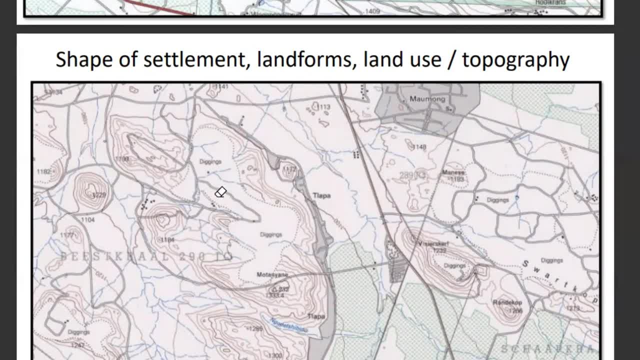 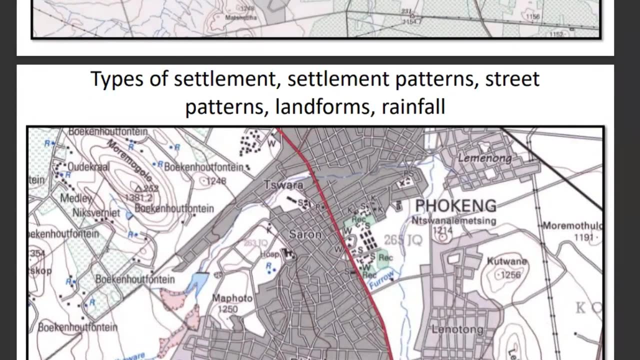 see a lot of settlement. actually, you must know that these are settlements here, so if it is concentrated in one place, it's nucleated. if it is dispersed, or it if it is, they are spread away from each other. it is um dispersed. okay, now, besides that, learners, we have also the interpretation. 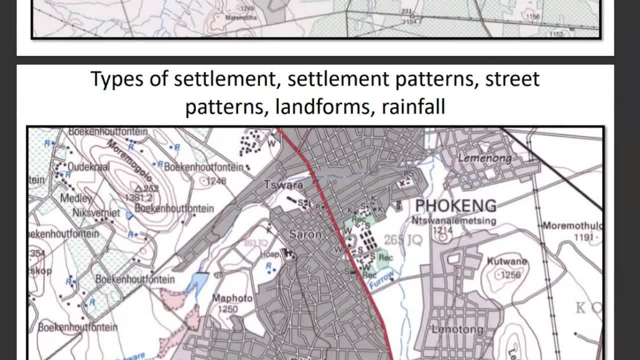 in relation to the settlement types. okay, we say the settlement types, that is, rural or urban settlement. then, besides that, we have the settlement pattern, which we said, that it is either nucleated pattern or or nucleated, which is the same as clustered, or dispersed, which is the same. 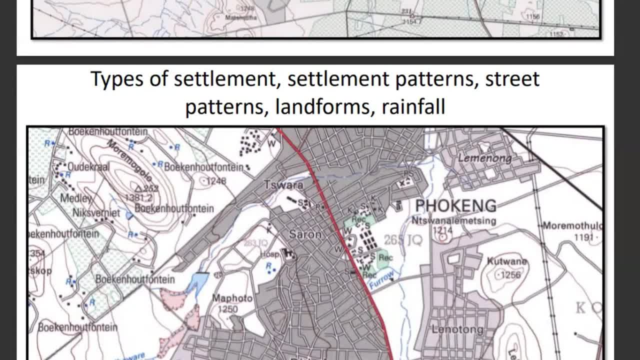 as spread pattern. then you have the street patterns. we'll talk about street patterns. what do we see? we're looking at the way the streets are being arranged, okay, and in this case, what do we see? look at these letters. we know that in our settlement, you must have looked at what they call. 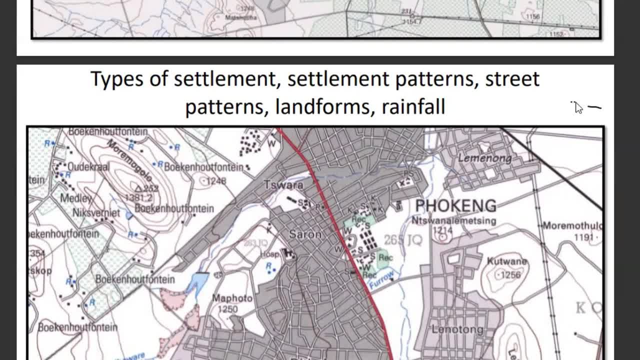 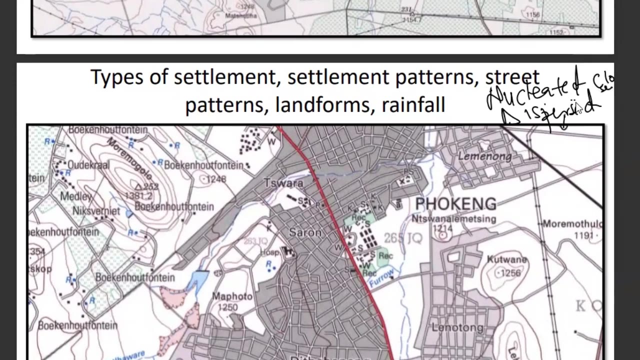 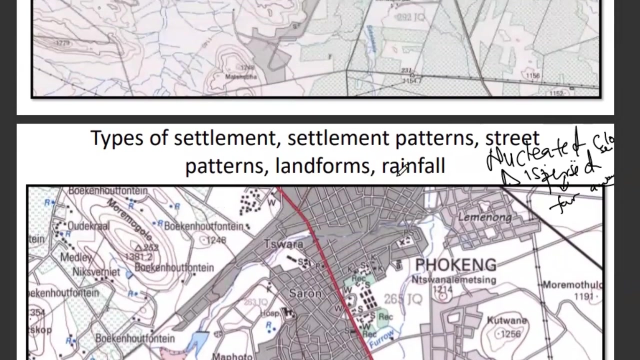 okay, in terms of settlement pattern, said we have nucleated, okay, then you have what you call dispersed and we'll talk about nucleated settlements close to each other. then here is settlement far away from each other, okay, so if you check on the map, do you see anyway where the settlements are so close to each other? 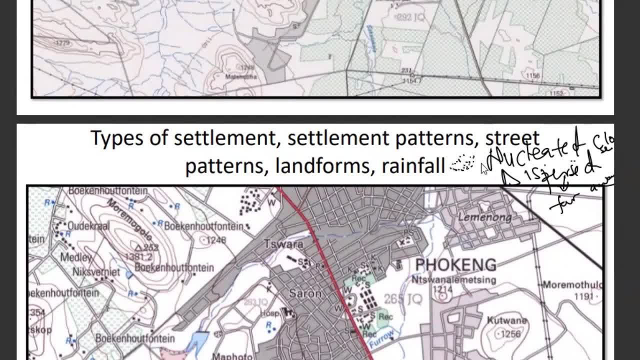 in one area like that, so that one is going to form a nucleated settlement pattern. what about this part? this part is going to form something like this: when they are spread from each other, okay, that is settlement pattern, then the street party, street pattern we have, basically, there is a grid. 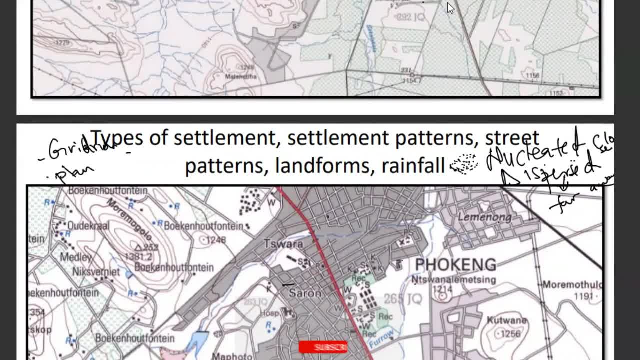 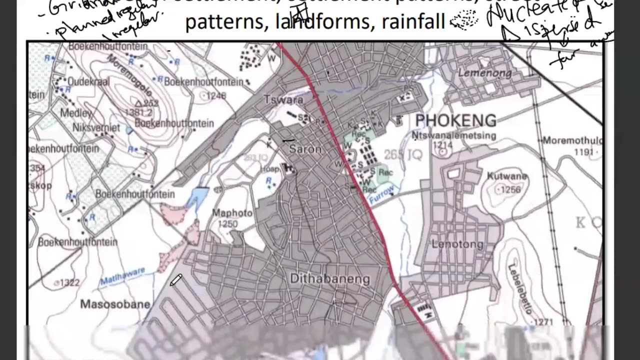 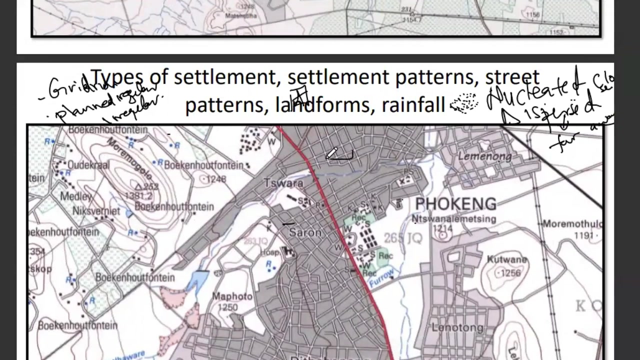 okay, we have planned, but planned well, planned regular and planned irregular. okay, then in this case, if it's gradient, it forms kind of grids, squares straight, and normally it is one way. so when you check around here, what do you see? you can start list here where they form a. 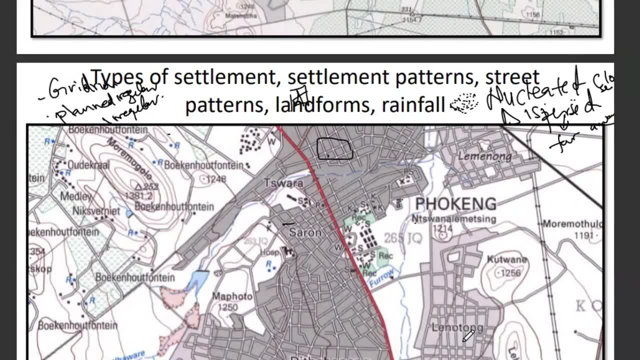 grid line in front of you. that's all you can see. you can start list here where they form a grid line pattern. see that, okay, and see maybe around here on the grid pattern: okay, then these other ones, like this one is planned irregular. then you have that one that is not having a proper shape. 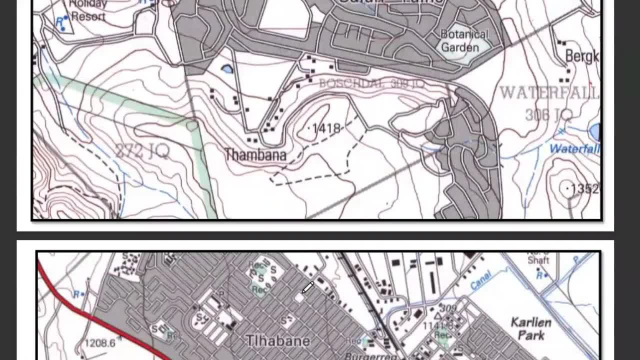 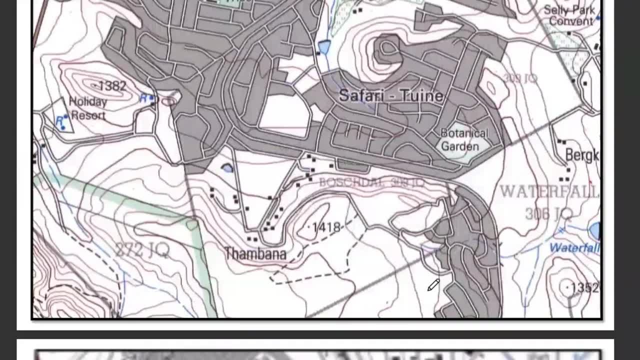 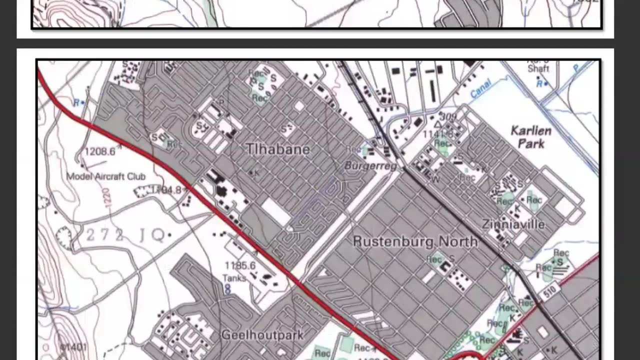 where the settlements are just spread out like, and the roads are just put anyway, so that one is irregular. but when you check there you will see that there is one which is planned, there is one which is grid and one which is a irregular or planned. irregular and planned. regular check here. 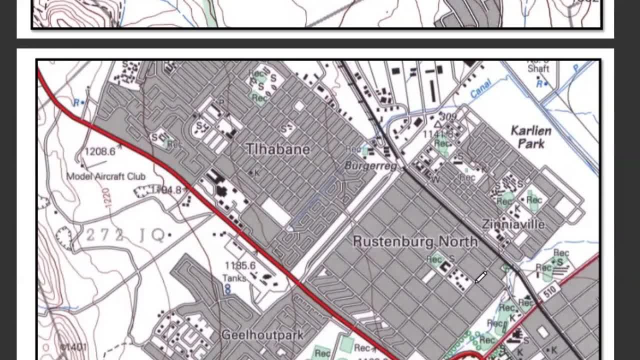 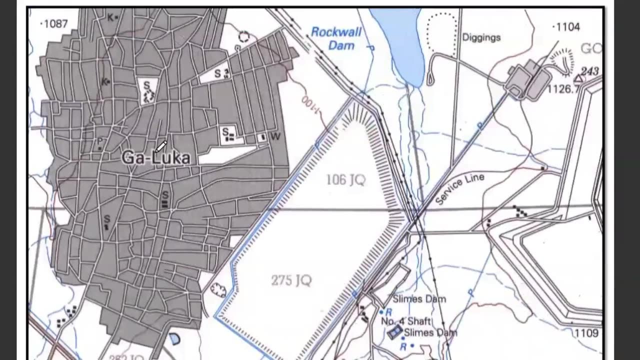 this is a very good example of grid street pattern. this is a very good example of grid street pattern. it's a very good example, planned, regular, but if it is irregular, it simply means it is not making a proper shape. take an example: this is unplanned street pattern because the way 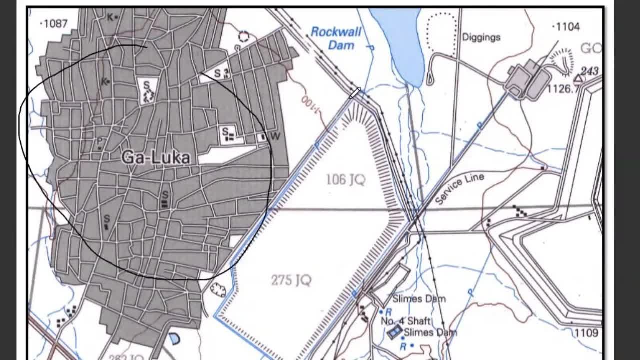 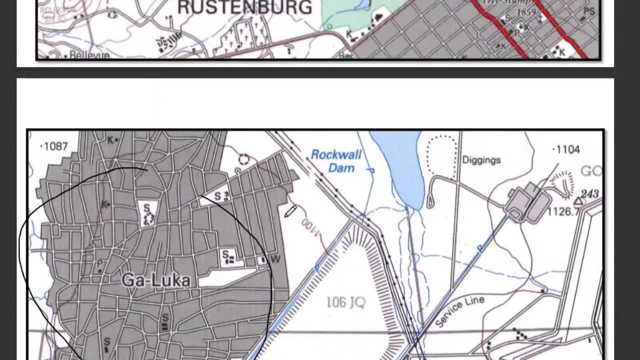 they appear, streets are joined anyway the way they want them to be. so that is interpretation of settlement. you are applying the concepts of settlement. and that settlement concept, remember it, is coming in paper one, i mean in paper two. and the economic geography is also coming in paper two. 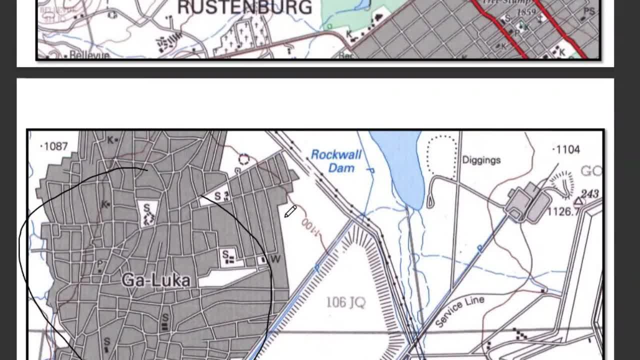 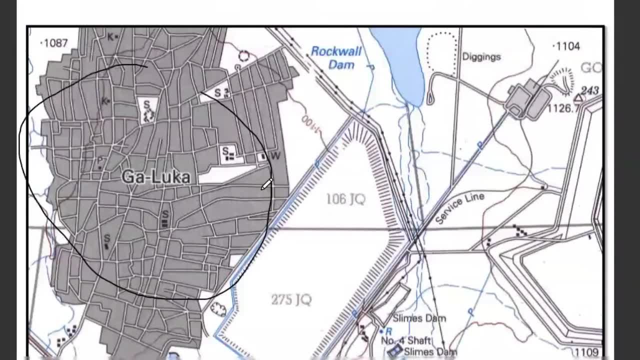 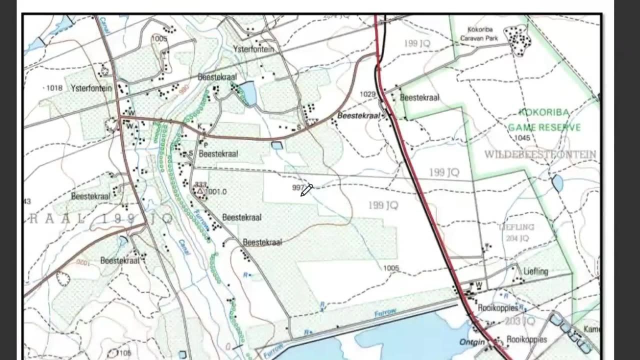 so climatology and geomorphology is the application that is coming in paper one. so learners get ready for those aspects been positioned to interpret them and then life moves as we expect. okay, now, like i've been telling you that we have a lot of things to apply, 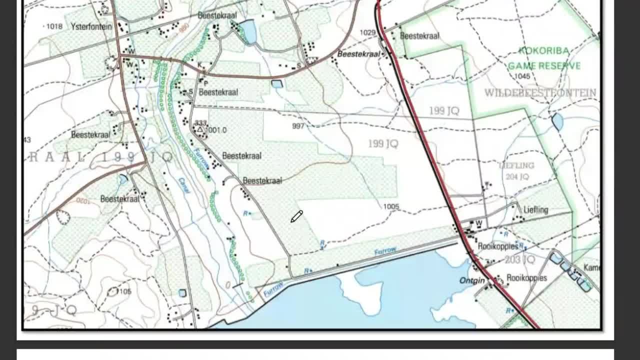 we have those areas that are flat, we have those areas that are steep, and how are they applicable? how are they important? if you look, here we have files, here we have canals, we have rivers. what do they all do? they all provide water for the farmers. okay, we have the 아이�ינו cincan. okay, you can apply ma carte in-game. you can apply money. 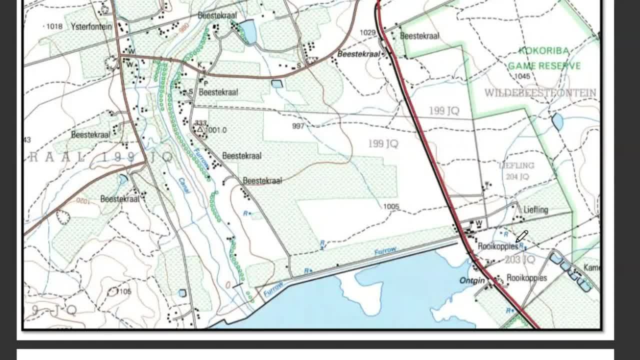 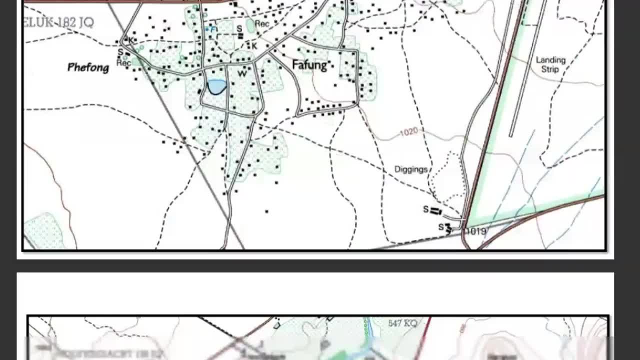 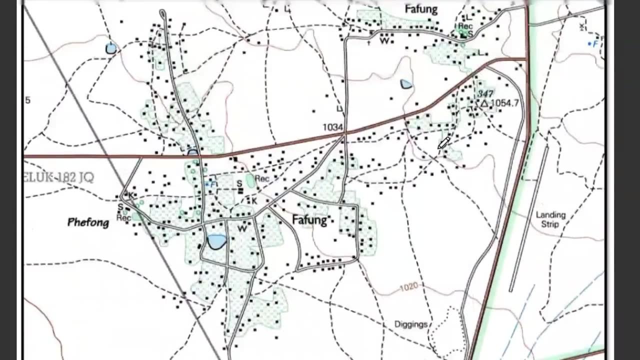 so you can pull it out. okay, the dams, they also do the same. they store water that is used during the dry season. okay, so please, i'm trying to show you some of the aspects. now we can also apply another concept somewhere here. i want you to look here. 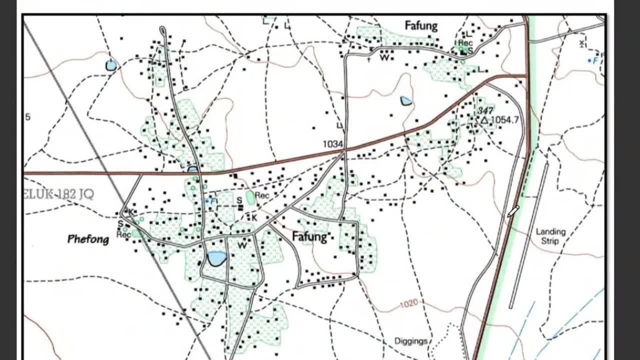 this place here because of the nature of the contour lines. it simply means that it's a bit gentler and that means a gentle water plant needs to be dried night sown- night in the case of hoop is okay- and that means a gentle slope encourages the development of transport routes for easy. 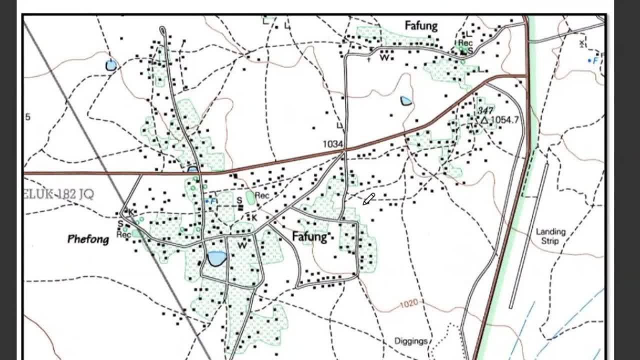 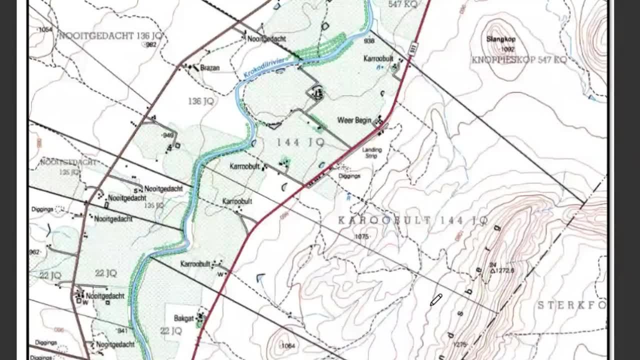 accessibility. now check here: a lot of roads that are running around or running around this area because a bit flat. i want you to look at what is happening this other side, because of the nature of the contour line somewhere here it is very steep. therefore, because it is very steep it. 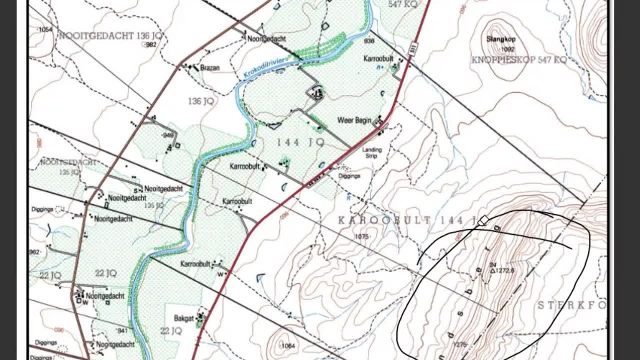 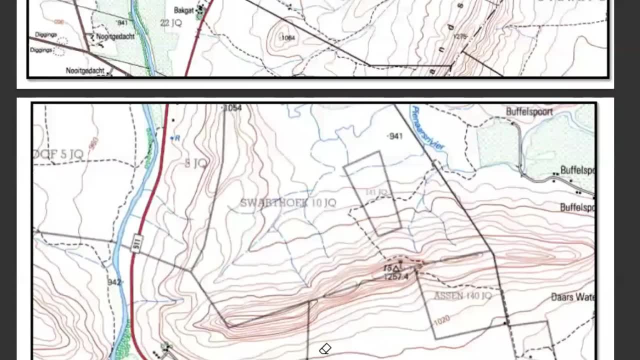 discourages the growing, the construction of roads, and the same thing that applies here. okay, that's why you see there are no more many roads here. if you check the only road that is here, it is passing where it's a bit gentler, in other words, between the two high lying areas. you see there's a mountain. 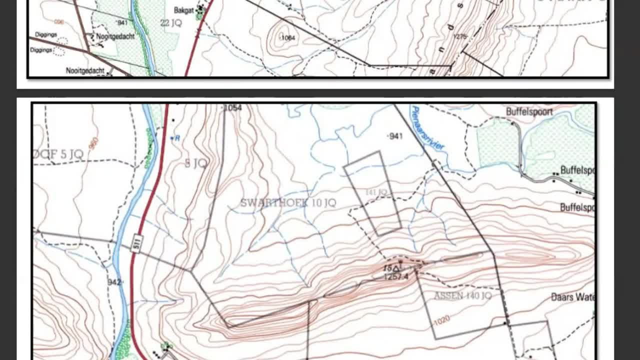 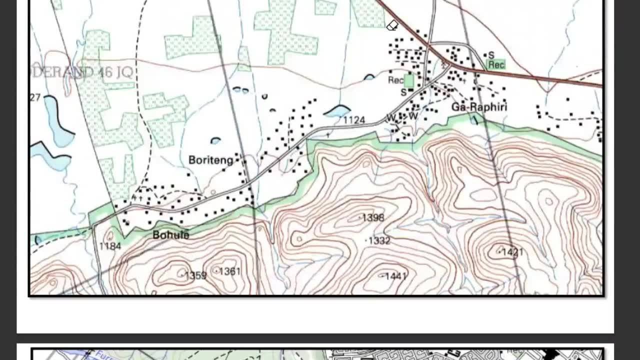 here it's a mountain, so this one, we shall call it a pass, okay, or a gap where the roads are passing okay. now you can see that this road, maybe it would have a chance to just go come direct through here if it wants to proceed, but it couldn't. why? because of the existence of the steep area. 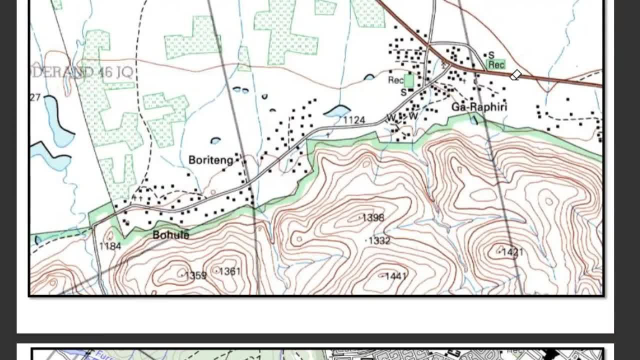 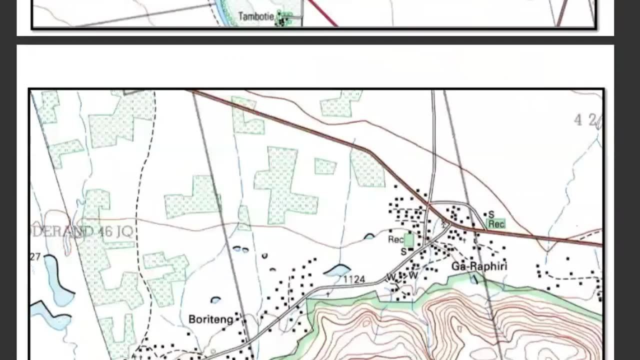 therefore, the road tries to pass around so that it can connect to other areas, because those deep areas are very difficult to construct roads onto. so hope, learners, you understand. okay, we are still looking at interpretation. whatever that i see that is really important for interpretation. i will please try to explain. okay, there is another aspect that i also want to. 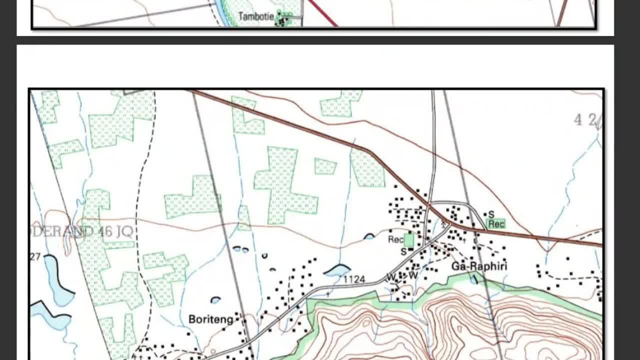 talk about that is related to interpretation, that is, the direction of the rivers and the direction of the rivers. okay, okay, let me start from the direction of the rivers, the action of the rivers. i want to use this river here. now you can ask what is the direction of? 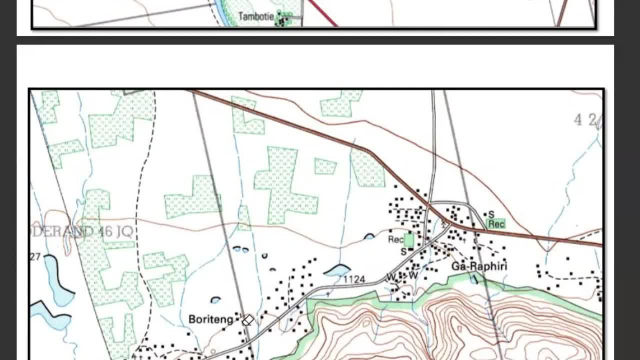 this river here. okay, i might not be having a name for it on the mean left hand side. okay, so your name for it in my timings야 bismuth, but maybe it will have a name now. let us use this as our example. where does the river flow? 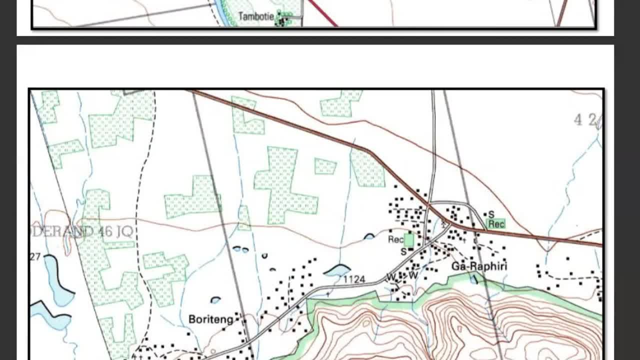 to do? you think this river flows from the north to the south, or it flows from the south to the north? good of thought, but in real sense this river is flowing from the south to the north. why? because of the dam wall. it's not having tributaries. look at the dam wall. the dam wall is this side and this. 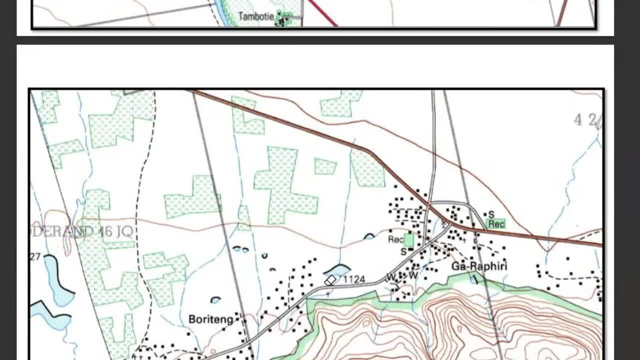 is where the dam is, meaning that the water is flowing from here, then, through the dam wall, it goes north. that is number one. number two: which other evidence do you have to show that this river is flowing in a northerly direction? is because of the nature of the contour lines or the gradient? 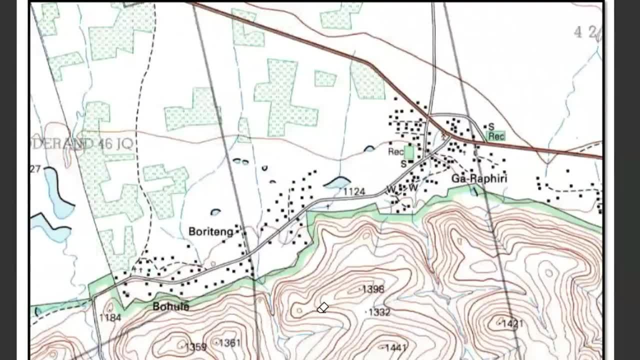 check here. you see, here, here is steeper, here is flatter, meaning that the river flow from a higher lying area, no lying area. so this river cannot be flowing from this way, entering where it is mountainous. it can only flow from the side that is a little bit mountainous, going downwards, because, remember, a river is a flow of or is 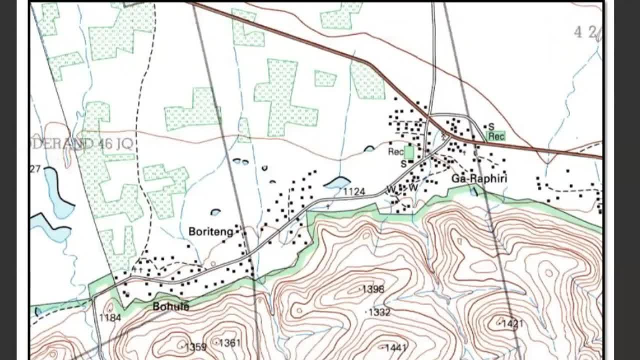 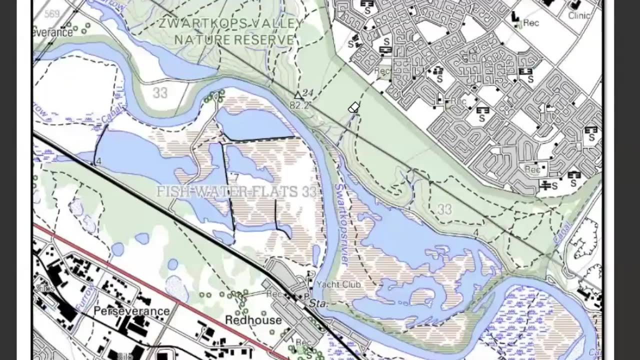 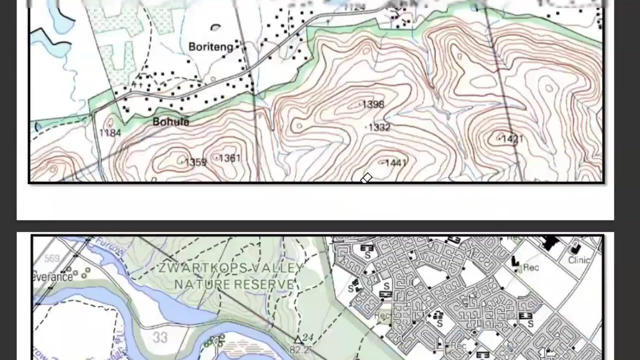 water that swiftly flows from the source to the mouth under the influence of gravity. okay, so this river cannot climb the mountain, and the river flows from a higher lying area to down or to downer areas. now, um, besides this, there is something that i want us to apply. still, look at this. this is the other. 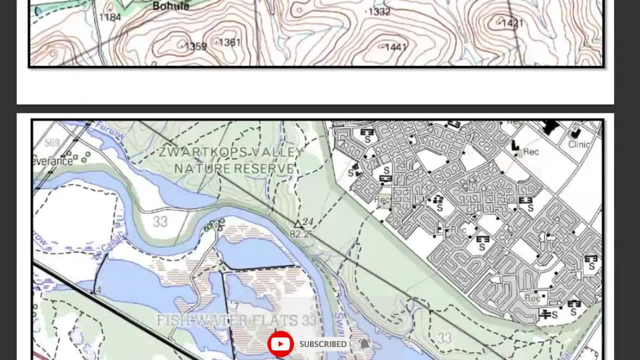 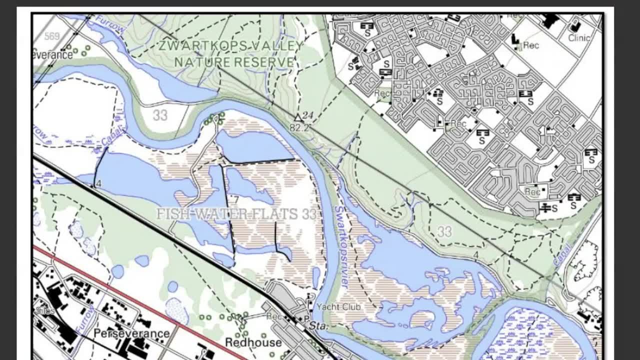 part here. when you check that part, which stage of river do you think? which stage of the river you think this river is called? what swatco, swat copra's river flowing to? where does it flow to? and then the next question can be: which stage of this river? and then they can also ask some 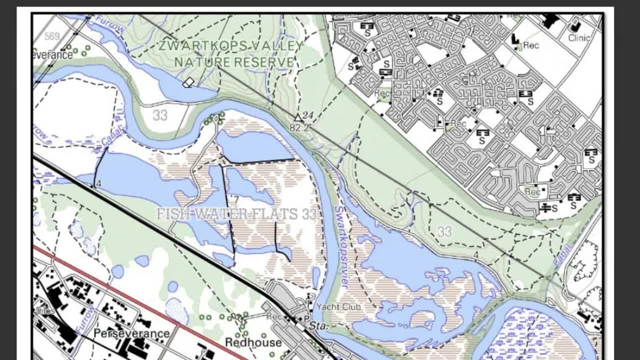 related aspects of one. they can assume the aspects of um uh river, buffer debuffling or the buffer zones. but before i reach the, let us start from here. when you look at this river here, look at the way the shape the pattern is forming. it's forming this meandering pattern and besides that, we look at the. 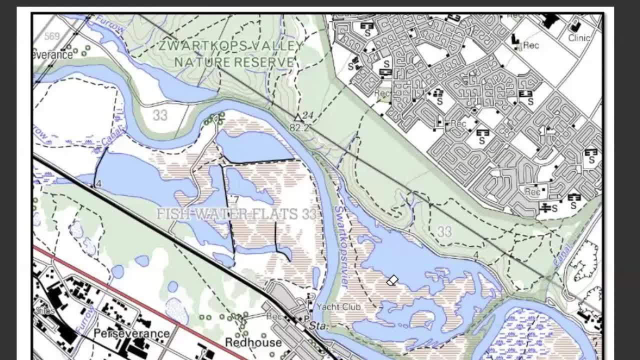 nature of the contour lines. it's not that so steep and it is not so that's so flat. so when you look at this area, we understand that this river is in its last section, it's in the last course. so if it's in the last course, this is what we call meandering. okay, and remember, in the meandering, 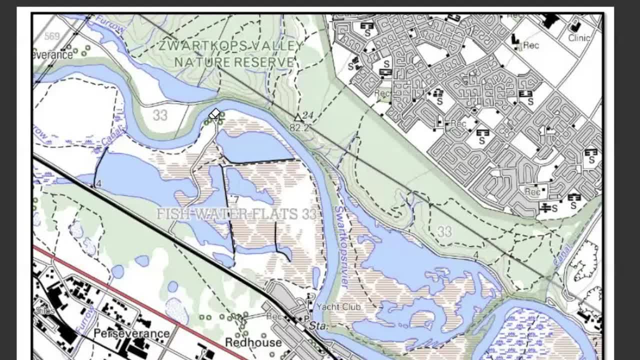 sections. there are some. there are some aspects we looked at if it comes to meandering, remember, we looked at aspects like what we looked at- aspects of meandering. then we looked at issues of the slip off. then we looked at another issue of the undercut and we know that if we talk about the undercut, what are we referring to. 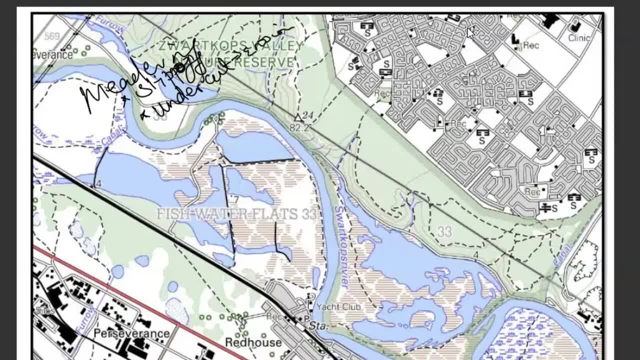 we are referring to the area that is experiencing erosion. we'll talk about the slip off. we are Referring to areas that are experiencing what Deposition, Meaning that the slip-off is what we refer to: the outer to the inner bend, Inner bend. 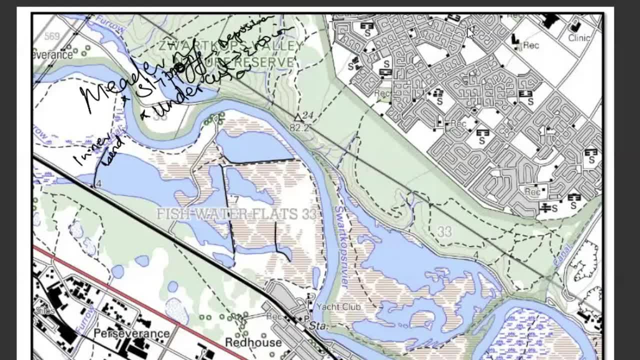 And the undercut is what we refer to as the outer bend. Let us check on this river that we are having. If you look at this river that is flowing like this, Meaning that as it keeps on curving and bending, we have the inside part, which we said is the inner bend. 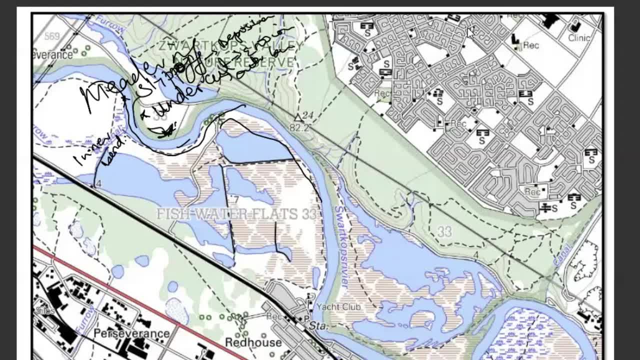 Therefore, this one is formed by deposition And the outside bend, which is formed by erosion. So outside is erosion, inside is deposition. And you know, when you talk about erosion, what do we expect? We refer to the fast-moving water, fast-flowing, sorry. 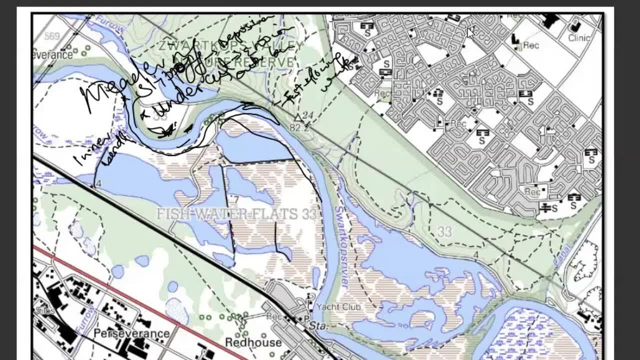 Fast-flowing, Fast-flowing water. Then we talk about dominant activity is erosion, Okay. We talk about the gradient being a bit steeper, Okay. And then the velocity: high velocity of water. Then, when we talk about the inner bend, what do we expect? 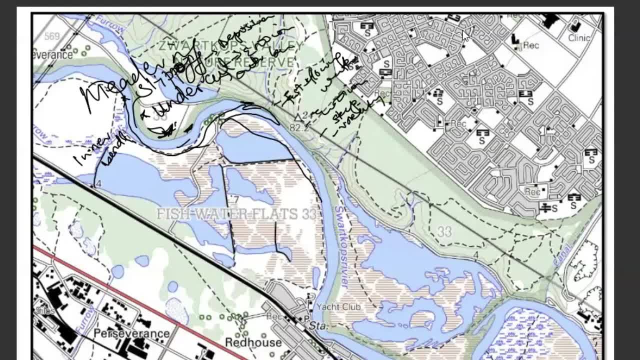 Gentle gradient Here. Here, You expect a gentle gradient. Okay, You expect. You expect aspects of deposition, Slow-flowing water, Slow-flowing water And then less velocity, Meaning that the inside bend. we expect slip-off at the slope. 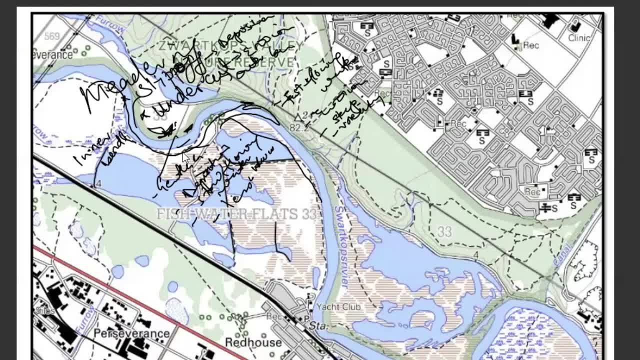 And therefore there is slow-flowing water, more deposition- okay, and the outer bend, which we said is an undercut, that's where we have water flowing faster and we expect the erosion to take place. the area is a bit steeper, that's why water is flowing faster and that fast-flowing determines also the velocity, okay. 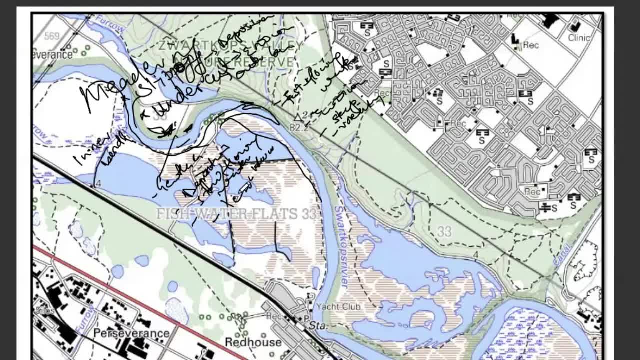 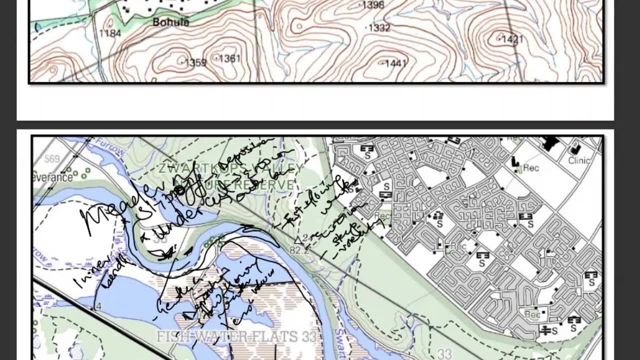 So that is what we refer to as meandering or a meander. So a meander, Meandering is a landform, Meandering is a process through which that landform of a meander is formed. Okay, So when we check, 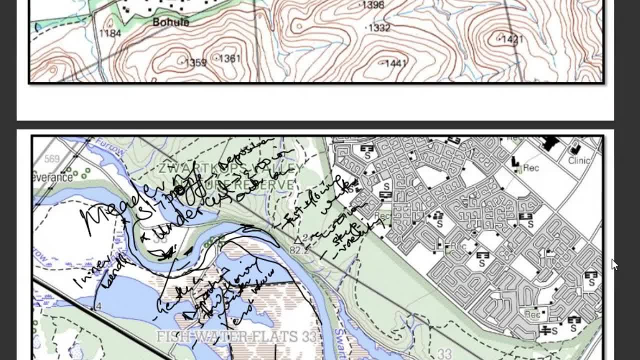 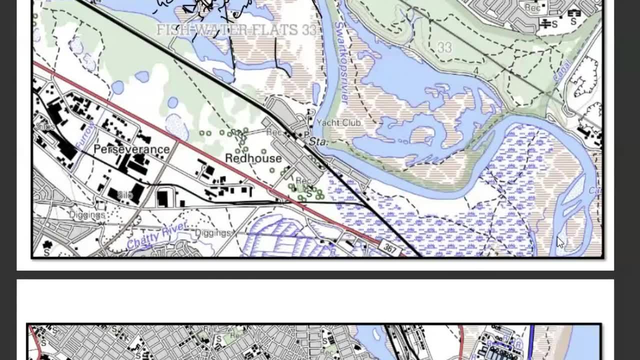 somewhere here we can still see another feature. Which feature is this one here? Okay, The feature that we are seeing here in this area is what we call a braided stream. What is a braided stream? This is a depositional feature. 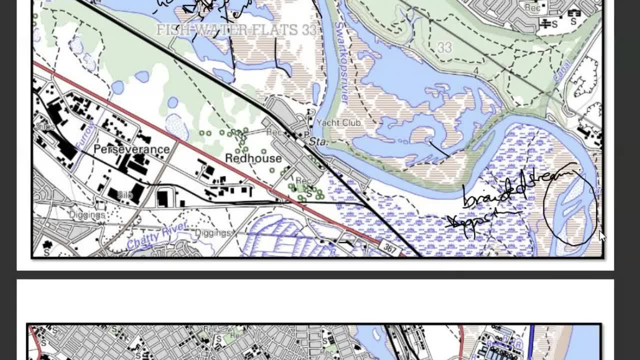 Its a depositional feature that forms when the materials are deposited in the river channel Are deposited in the river channel, Okay, Meaning that since the device in its last stage, it means it has got less power to erode, less power to erode. 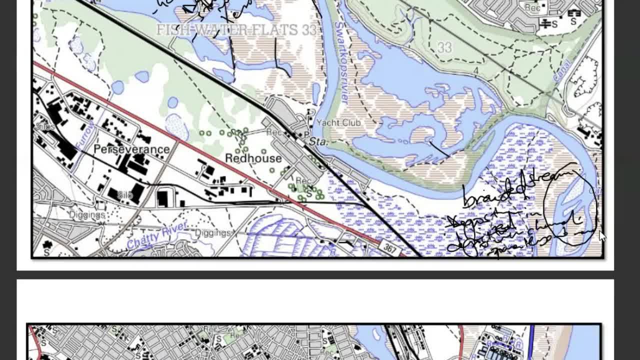 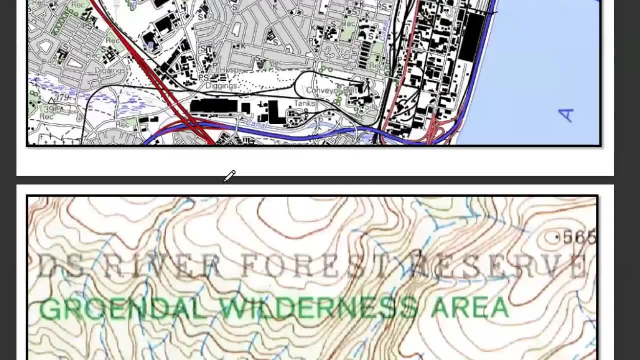 okay. so if it has got less power to erode, that means it dodges the material and later reconnects. that's why you see this river is flowing like this. so this one dejoins, this one rejoins, and then the river keep on flowing to another destination. okay now. 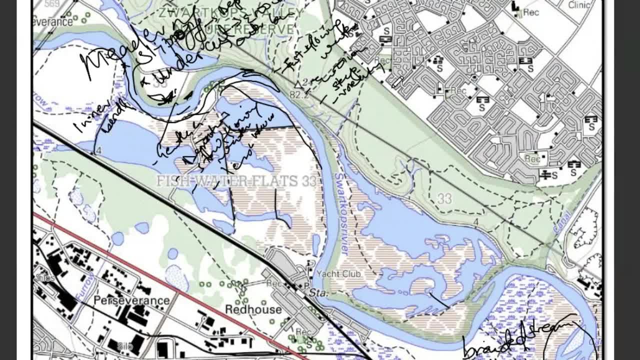 that is what you call the braided stream, so the area that is adjacent to the river, this part here, is what you call a flood plane. okay, is what you call a flood plane. so, learners, you can be in position to interpret those aspects. you can see that somewhere here. 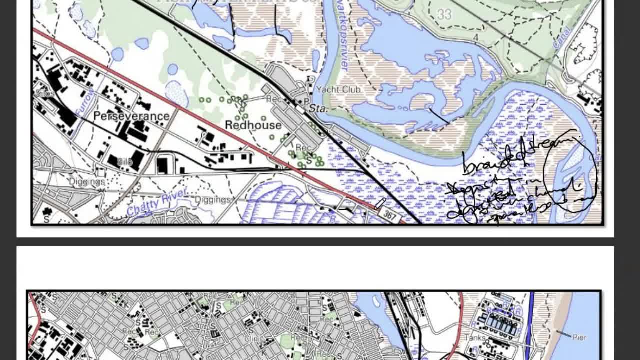 is flat. that's why you see the areas. but even the marsh unveil because the area is flat, it's having a lot of water that is sitting in that area. okay, remember learners, don't forget we are still looking at interpretation and i am trying to to put all the topics in the 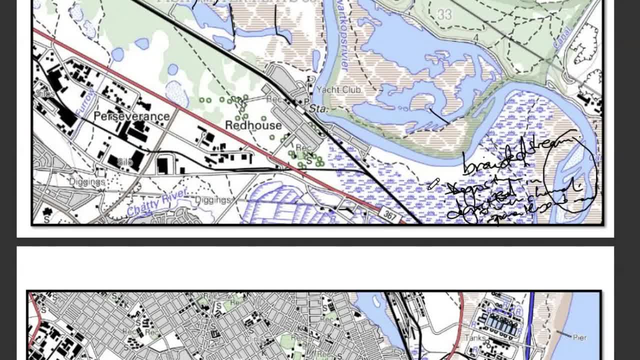 geography syllabus all together so that we can see how can each concept, or how can the concepts, be applied on the map. Okay, If you see anything that you're not understanding, please feel free to ask questions or to leave a comment. 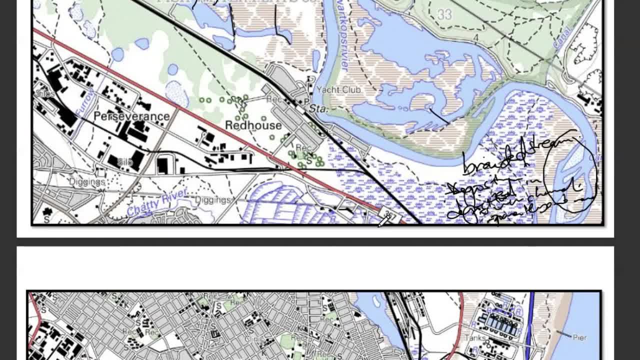 I'll be in position to answer you Okay, But in preparation for exams, please take note of everything and let us try to pass Okay. Now, besides this, there are some other interpretation concepts that can be applied. Take an example. 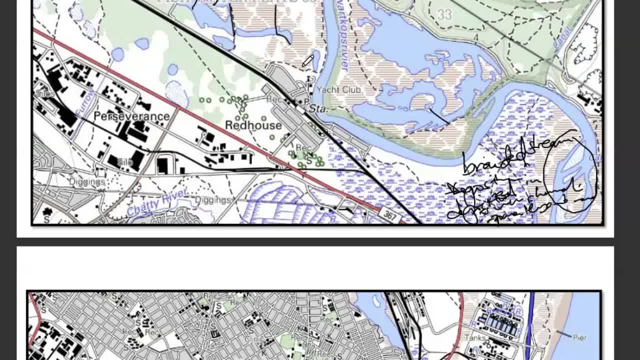 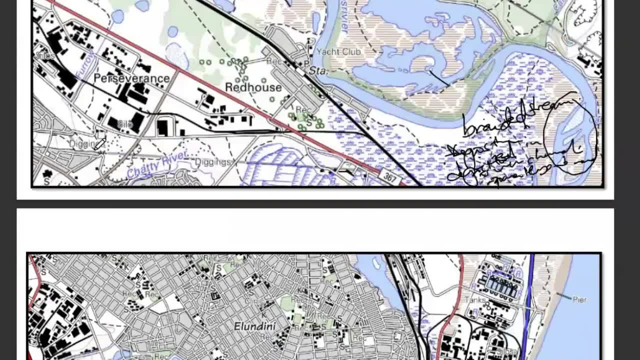 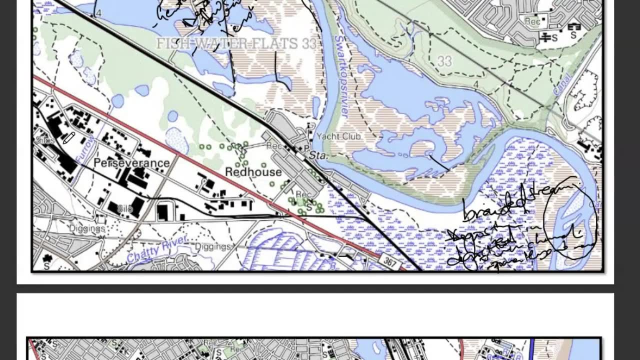 There is this area here that is a bit far away from the residential areas. Okay, This area has got very big buildings. It has got even the zeros. What do zeros do? Those are the ones they use to store. Those are the ones they use to store agricultural products or food. 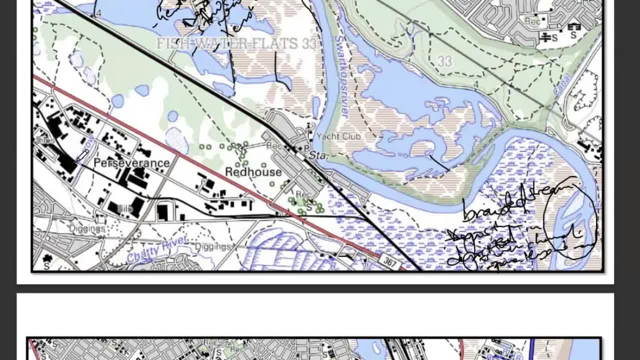 Okay, Now, when you check here, you'll find out that they are very big settlements. Yeah, they are very big buildings here. Okay, These buildings, we can term them as industrial areas, And we can. what do we remember when we're talking about industrial areas? 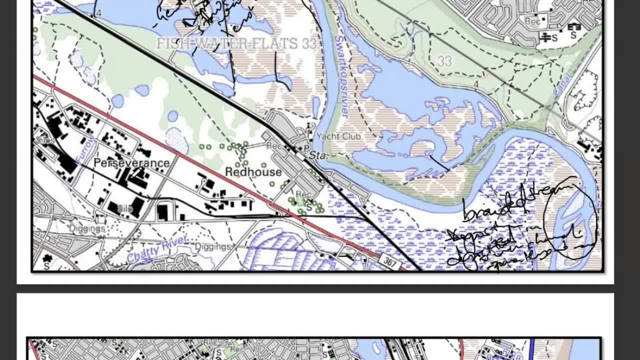 First of all, industrial areas are meant to be far away from the settlements because of the noise. Okay, Industrial areas are meant to be have stay to be in areas where the land is cheaper, is cheap and available like large areas. 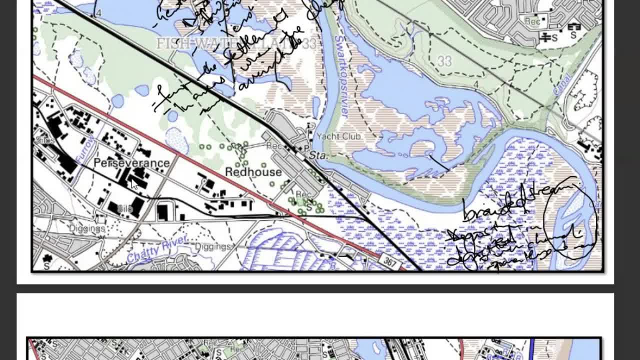 where those industries can be established. Okay, It is established close to the roads or communication lines, Okay, Which you can see, that there is a road here that is going, there is a road, there is a road, and so on, Meaning that this industrial area is basically, this area is basically an industrial area. 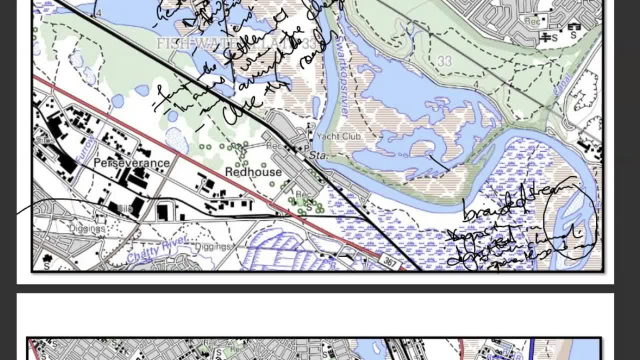 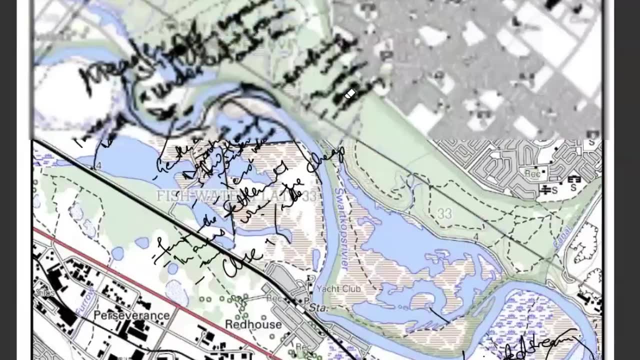 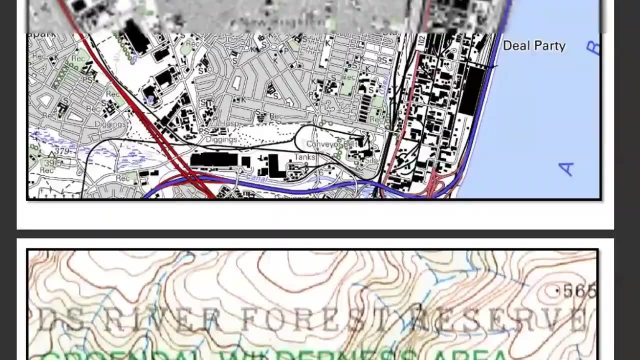 according to the interpretation of the diagram. Okay, Now, now I want us to proceed and look at, keep looking at other aspects. We are still looking at interpretation learners. I told you, today at least, I want to see the interpretation part. 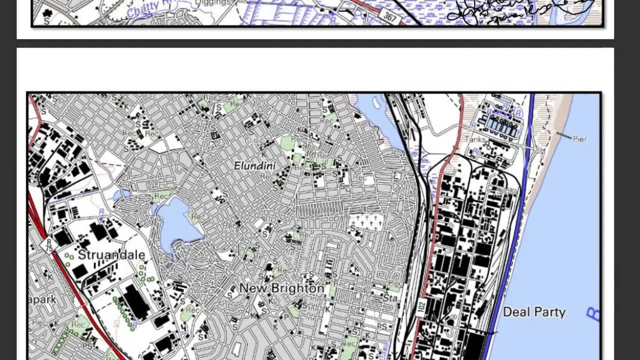 There is another time where I handled the calculations And I know that I finished all those calculations. If there is anything that is remaining, please let me know. I will re-handle it, But if there is nothing, we are still moving forward. 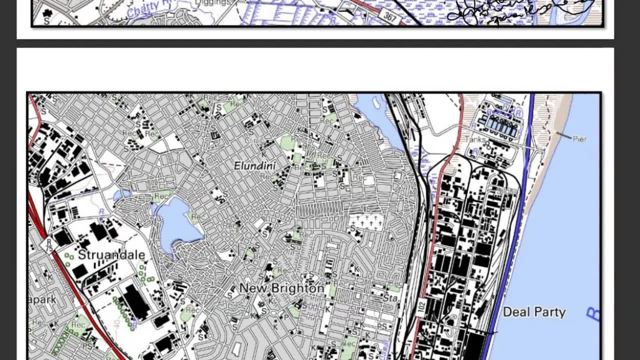 And apparently I want us to look at interpretation And as, as far as interpretation is concerned, we are almost done because we have looked at all the possible ways in which questions can be asked in relation to the different topics that we have looked at. 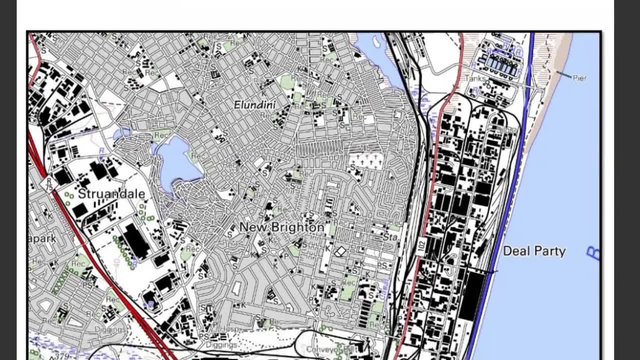 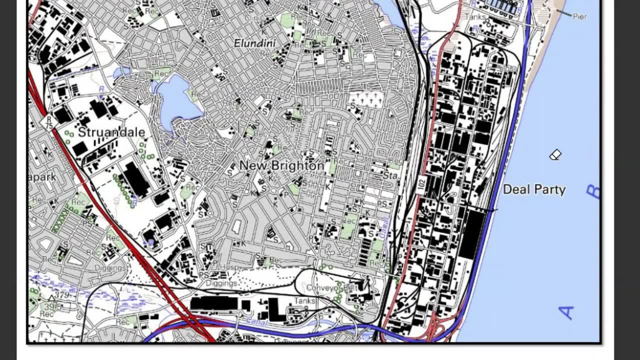 Okay, Now here we go. We look at another area here on the map. What do we see? Do you see somewhere here? these are industrial areas. Okay, Those are industrial areas. What do we remember? Like we mentioned above, 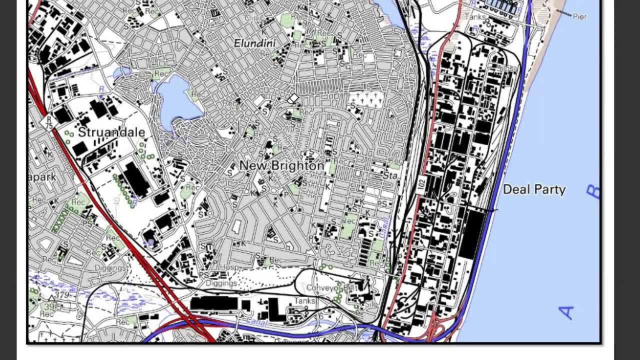 That all those industrial areas are industrial areas. They are industrialized areas. They will be built first of all next to the major communication lines. Take an example here: There is a road here, 102.. There is another one here. 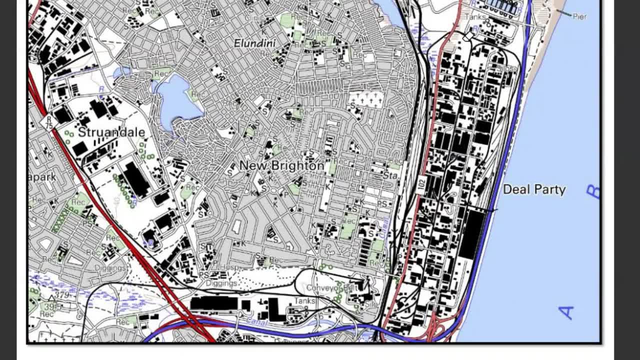 There is a railway line there. There are actually a lot of railway lines there. Okay, So these are industrial built up areas, meaning that such industries discourage people to settle close to them because of the noise. they make the noise pollution, So people are staying, basically, there. 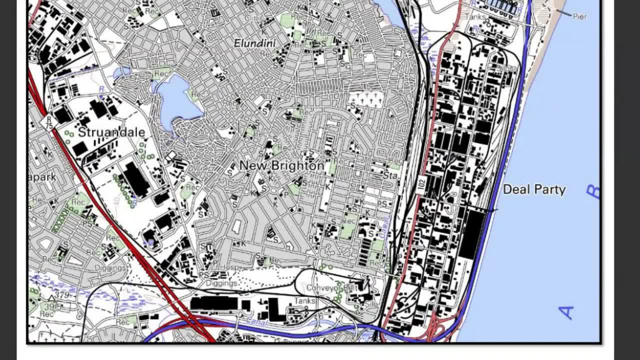 Okay, So people are staying basically far away from those industries. The reason why they are close to the main road is mainly because they need to transport- easy transportation of raw materials from one point to another and then they finish the goods Okay. So we can have a lot of factors. 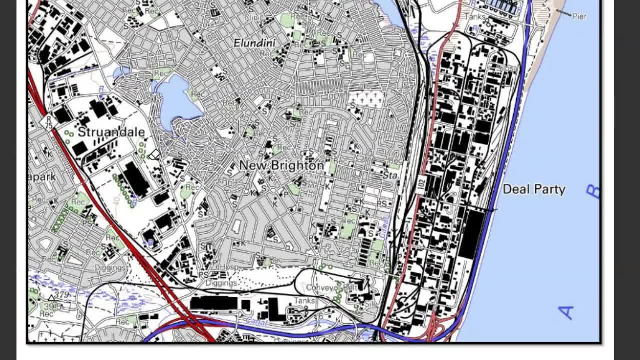 For example, some of the questions they can ask here, like explain, maybe, or give or discuss, or whatever- Two factors that have contributed to the development, The location of those industries, wherever they are. Okay, Maybe the industry is in a strained alley. 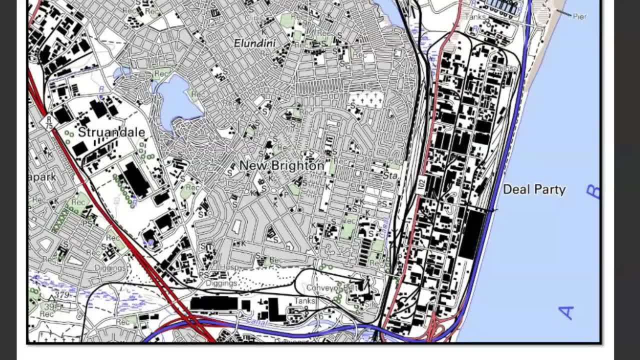 So what do we look at? We look at aspects like, for example, flat land, and you can see the area is flat because the contour lines are not so close to each other. Okay, That is number one. Then the very big space available. 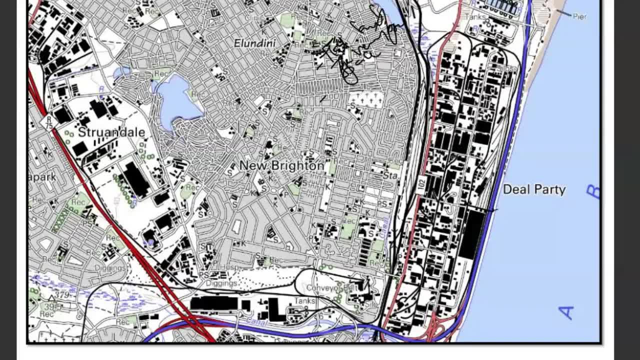 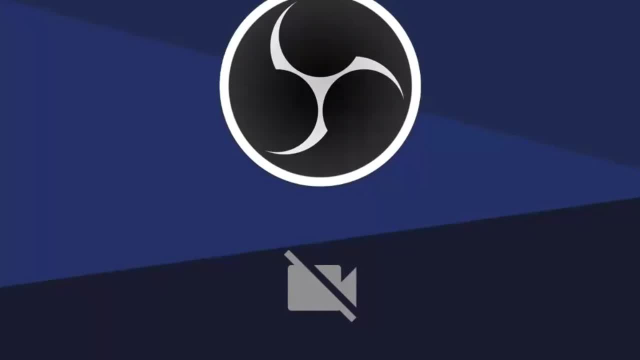 Very big space Available. Okay, For the expansion of industries. Okay, Then we also talk about the proximity or the closeness to the main roads. Okay, The existence of the main roads, The existence of the main roads. Alright, The existence of the main roads. 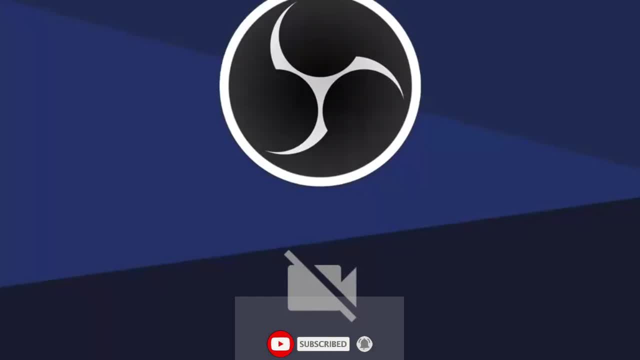 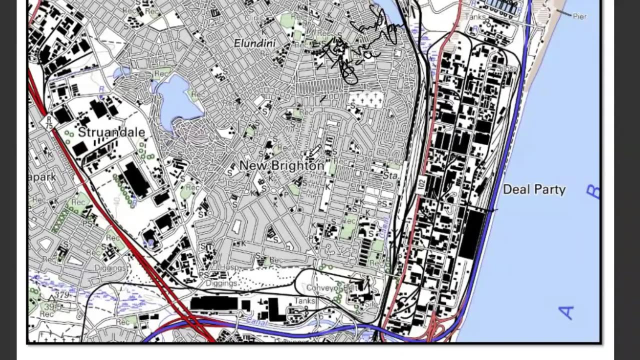 so those questions can be asked, that what are the factors that have contributed to the location of these industries, wherever they are? number one: they are far away from people. they need a flat area. they are far away from people. they need a very flat area. accessibility: the roads. 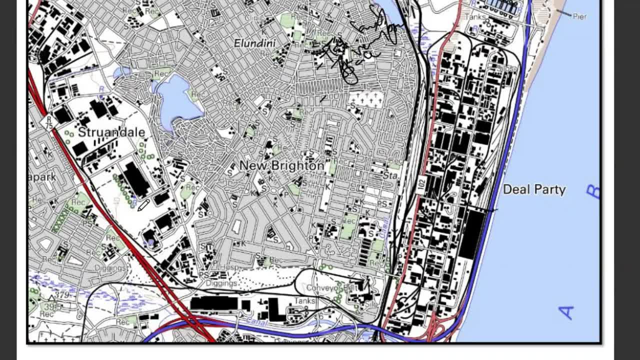 closeness to the water bodies or to the water for easy access to water. you understand um close to other residential ao and we are saying that the. the message that we are sending is that we are not going to be able to the. the message that we are sending is that we are not going to be able to. 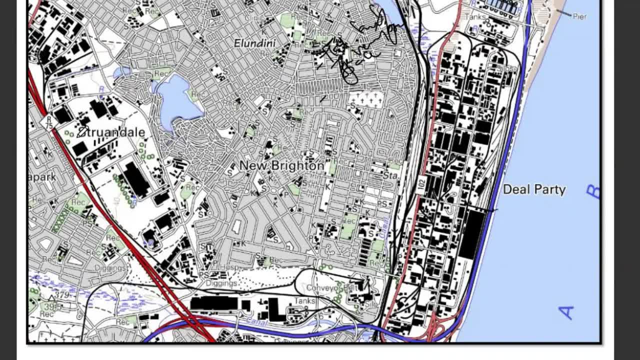 be far from people because it makes noise in the road, the flat area, the cheap land, a very large space for for their expansion, okay, and therefore we also talk about the capital that is basically needed from the nearby people or the cheap labor that they can easily access. so you can see that 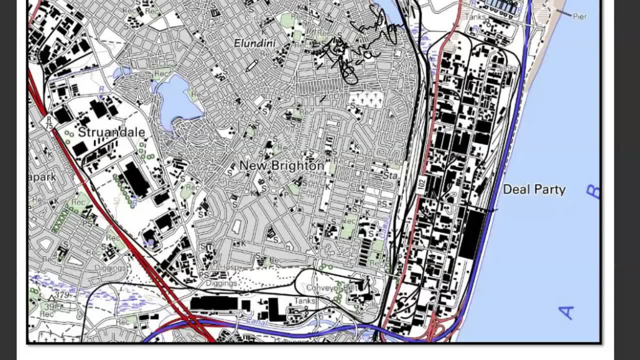 here is basically developed area. okay, it's more of a well-developed area here. then here is an industrial area. what do we notice here? that industrial areas are located and on the outskirts of the city, far away from the people. okay, and it is exactly depicted here. you can see these are settlements around here. this is a developed town. 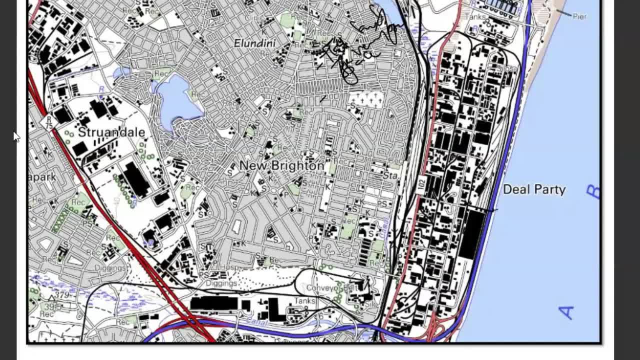 or a well-structured town, and then you can see that the settlements or the industries are a bit far away from from people. okay, now, those are some of the aspects and we can talk about there. okay, and it is exactly depicted here. you can see these are settlements around here. this is a developed town. 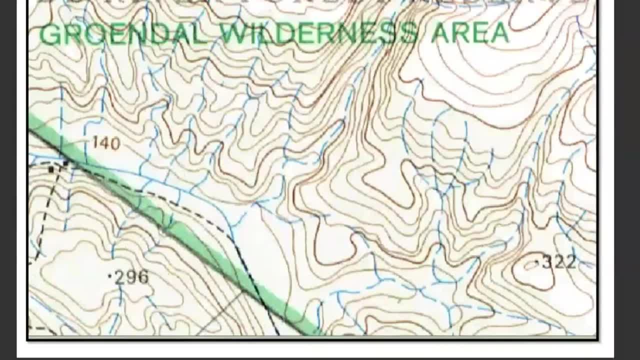 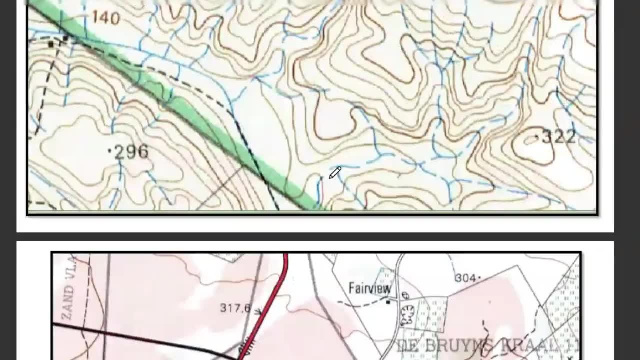 or a well-structured town, and then you can see that the settlements or the industries are a bit far away from the people. okay, now, those are some of the aspects and we can talk about there, okay, and we can talk about there, okay, these aspects of conservation. sorry, the aspects of conservation. 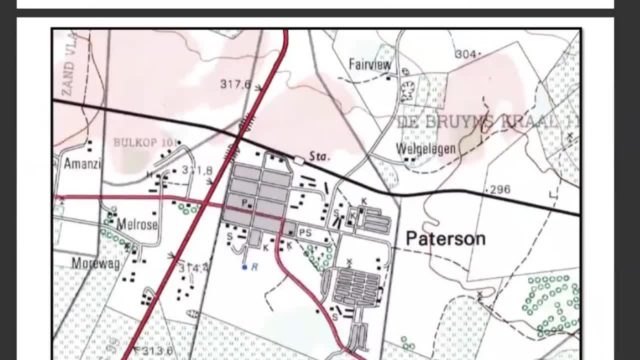 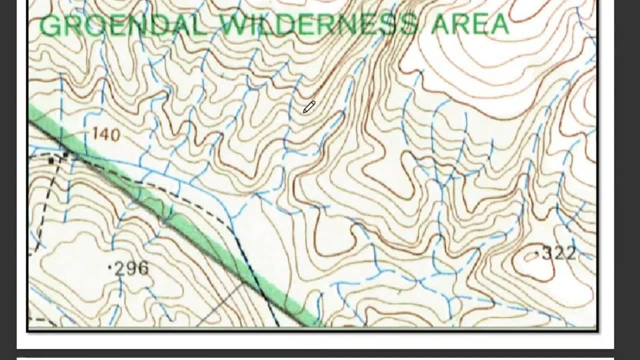 and the flow of rivers. maybe here i thought after seeing this, i remembered, here we can tell another, the way we can. another way we can tell the direction of the river is by looking at it, the angle at which the tributaries are joined, the main river. 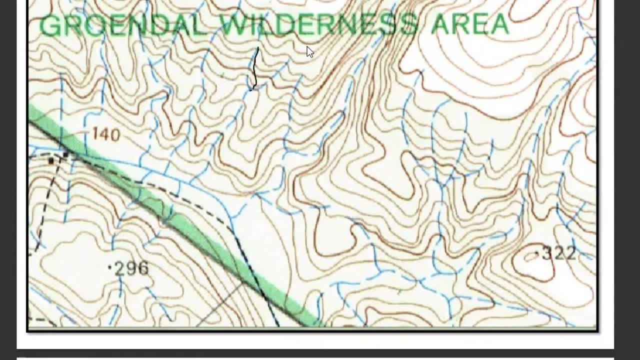 now, let's check here this one. now let's check here. this one is joining this one like this, so it is flowing to that extreme end. this one is joining like this: okay, so it is flowing. this way, you can see the way at which angles are joining, the rivers are joining others. 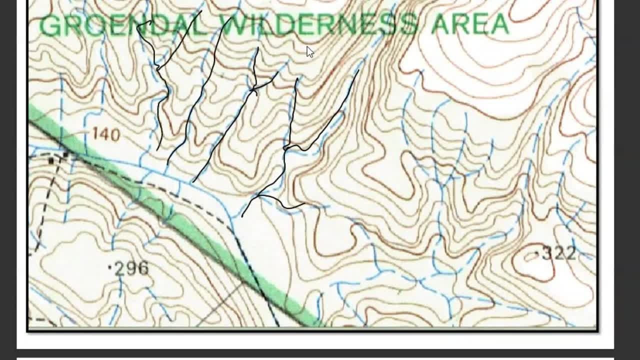 you can see this one, it's joining this one and then it flows downwards, meaning that these rivers are flowing towards this other main river and when you look at this nature of the river, there's another river there. so how does this river flow? how is it flowing? you can see it's basically going towards that direction, so it's flowing. 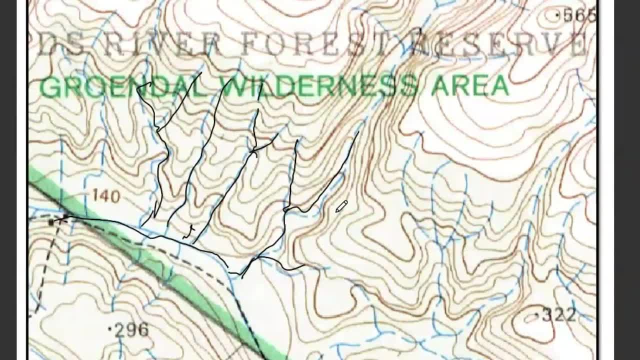 towards this direction. okay, so the angles you look at the v determines the direction to which the river is flowing to. maybe another concept that we can apply here is the concept of the stream ordering. look at stream ordering. we look at the independent streams, for example: one and one, it makes two. one and one, it makes two. one and one, it makes two. now, these are all. 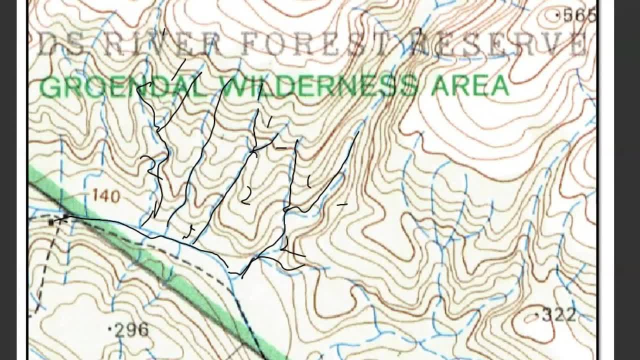 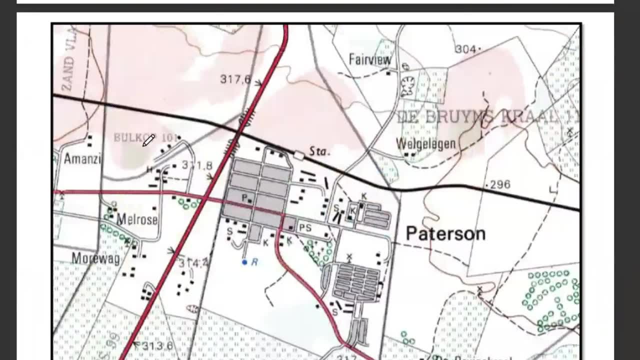 seconds, two orders. but we shall understand that clearly when you look at another clear diagram. okay, now, when you check here, you can see uh other symbols. now, if you do not know what the symbol means, this is the the right time for you to know. you still don't understand what this symbol means, what this one means, what this one means. 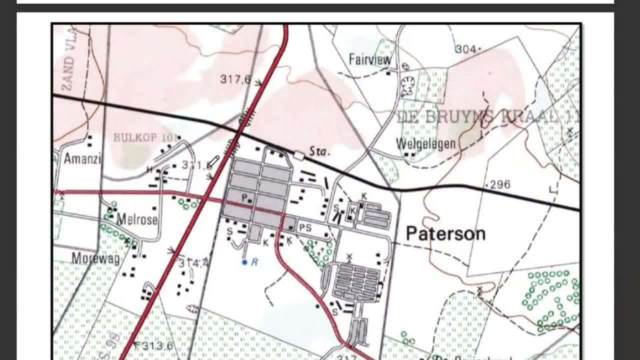 and so on and so forth. so you must- now- this is, when you look at this symbol- you go to the map and then check, okay, and then you check, and then you will understand that this symbol means this, this one means this and this one means this, okay. 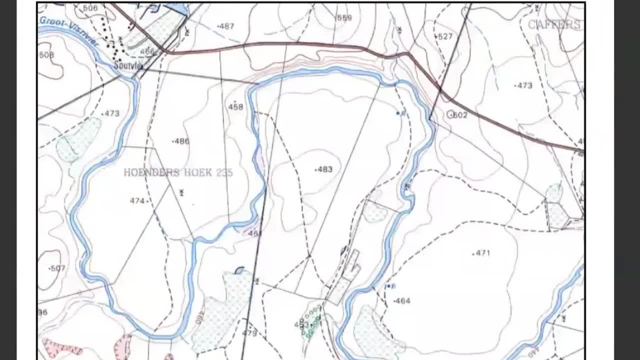 all, right now this is another, uh, another map that is trying to give us another clear view of the interpretation. you check that. you see that this river, river, karate here, grow to this, this river, fish river, is flowing in this kind of shape. so this kind of shape, we call it what? 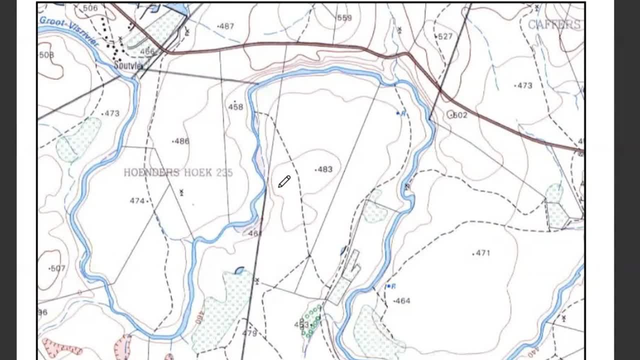 what you call a meandering river. so when you check this river, this river is meandering. so this one, if um, you remember the meandering process, say this is the carving and the bending of river. it happens in the lower section, or when the gradient is bit gradual, or latter and when 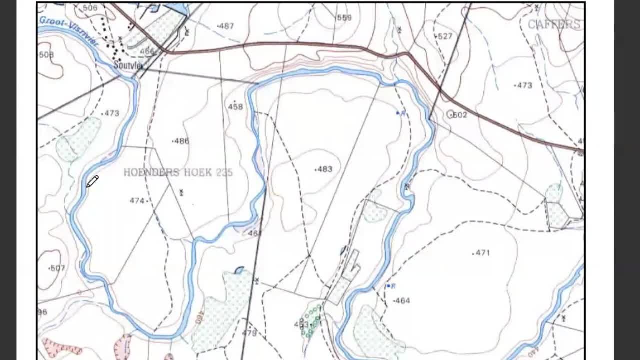 you check here, this kind of gradient is the same you see. so this river is flowing, carving and bending like that. remember, inside one is slip off, outside is undercut. so we said: outside is all is a steep slope, inside is a gentle slope. you can even see here the nature. 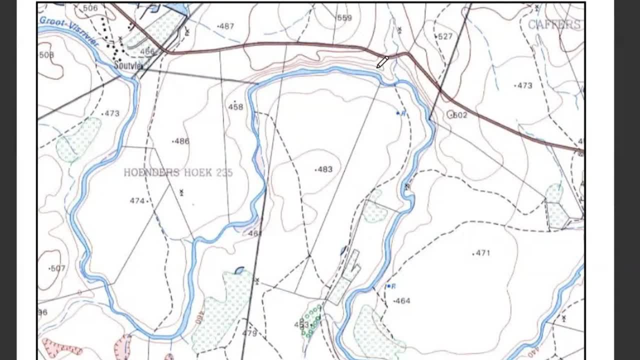 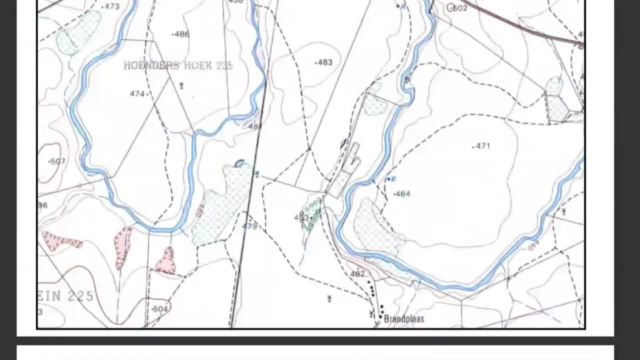 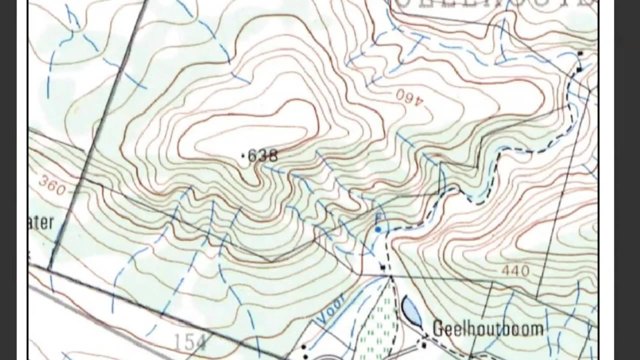 of the contour lines out here is basically depicting a steeper area compared to what is inside here. so that is application of another concept. now that this is now trying to assist us to get to know more other maps, how can it appear, please learn, has been positioned to tell. 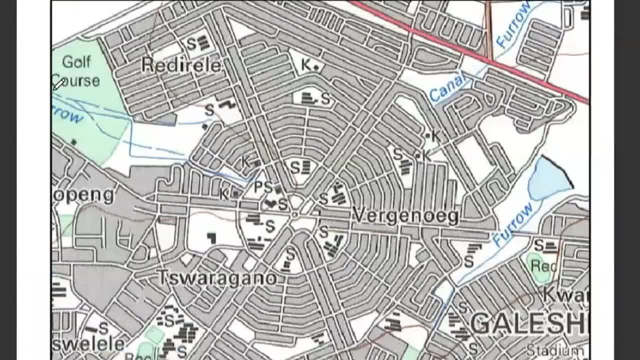 how it appears. okay, if you remember in your settlement you must have looked at this kind of settlement pattern. okay, this is what you call a radio settlement pattern, a radio street pattern? okay, radio means when the roads are radiating or connecting towards one central place. okay, if you. 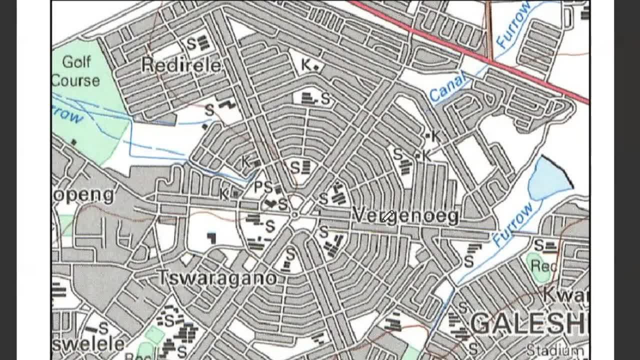 check here. this is a road, it's a road, this is a road, this is a road, basically a cobweb. okay, from a central place, okay, so this one forms what you call a cobweb kind of cobweb. so this kind of of settlement, or the nature of the streets, the way they lay, is determined by the main roads that are. 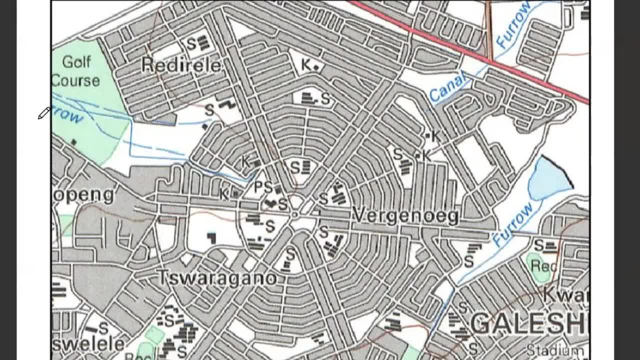 connecting the main central place. so here is a central place which is going to be our now cbd, that is having many openings of the roads from the nearby surrounding area, so those roads are all connecting towards the one central place. okay, so this one forms what you call a cobweb kind of 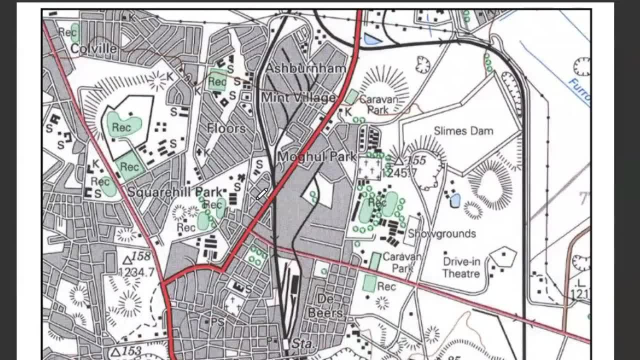 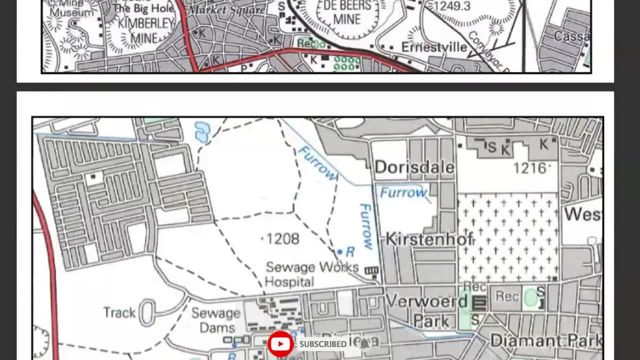 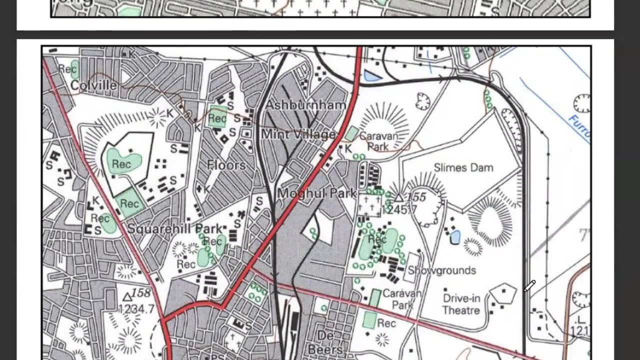 street pattern, okay. other activities, other interpretation that we can look at for the mind dump. you can see the dpa. you can see the roads- okay. you can see the roads here. okay, you can see the development of the town. you can see mining taking place around here. 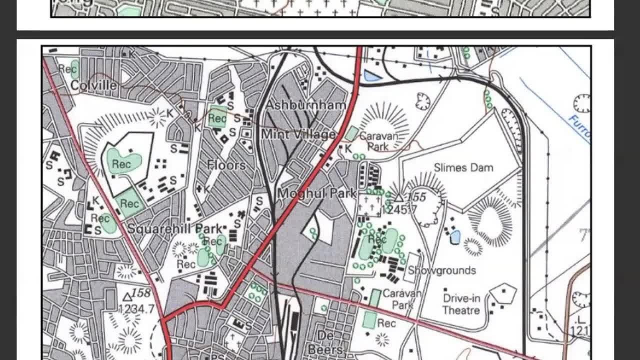 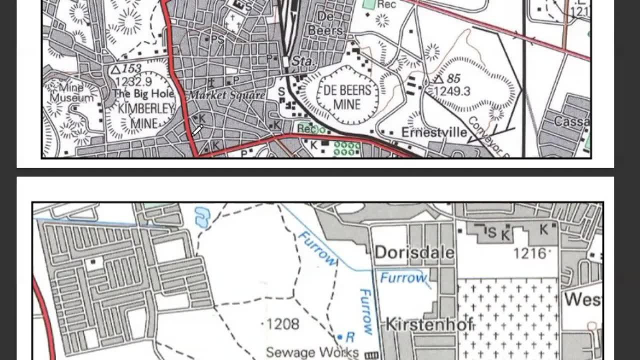 you can see drive in theater, meaning that there is entertainment taking place. so you know, that's the lot of things that we can interpret on the map. there is a mining museum, which now indicates that if it's a museum, it's basically promoting culture. okay, and then here. 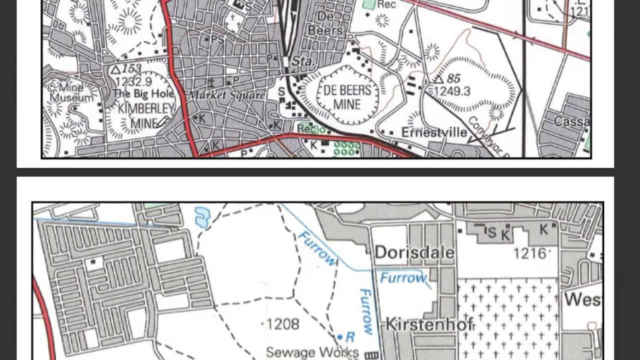 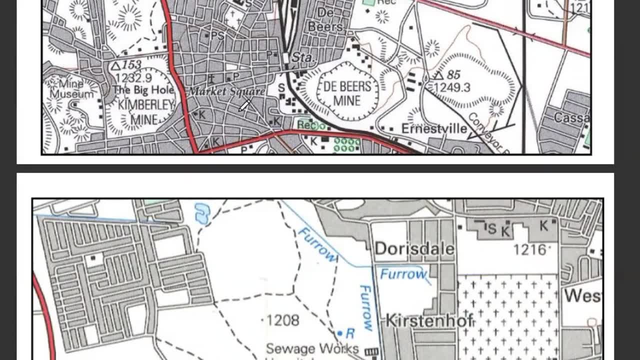 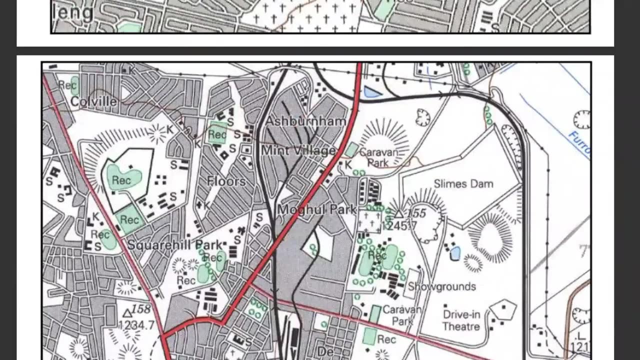 is what you call a big, whole kimberley mine. that means there's mining taking place. oh, there was mining that was taking place there. okay, so basically this is a mining town. if you remember very well, what we talked about in settlement, maybe with your teachers, is what you call a specialized 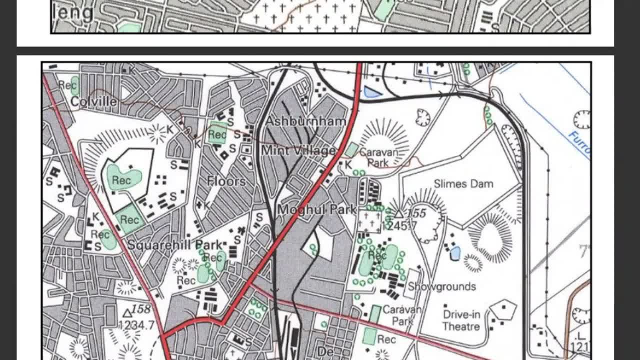 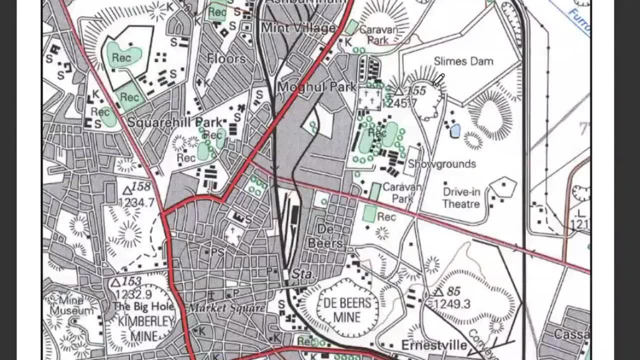 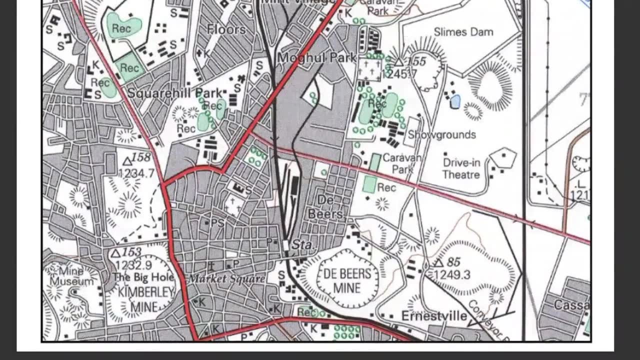 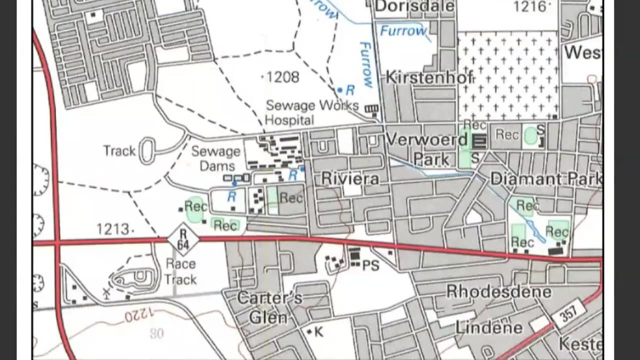 town basically doing one activity, for example, mining town. okay, and this way it's an example of the mining town to say so, because around here it's basically surrounded by mining only as the main activity. okay, now we still look at other aspects here. okay, remember, learners, it is nothing like i'm. i'm trying to. 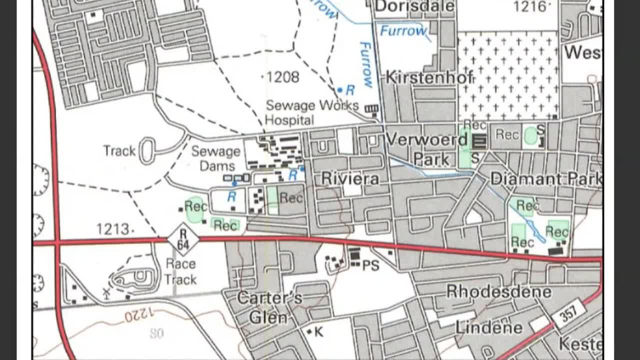 it's not that i'm trying to repeat these aspects, but i'm trying to show you that on different maps, if they bring you in a map from any area, you can be important to interpret, fast, oriented to the map. when you're given the map, check nicely and then, before you even check the questions. 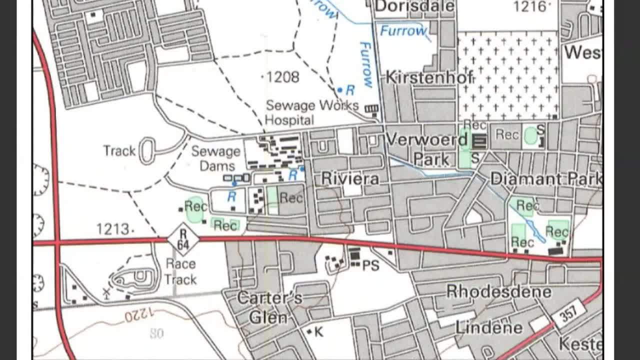 think of the possible kind of uh questions that can be um asked okay. so the possible kind of questions that can be asked depend on, maybe, how the map is okay. so if you oriented the map nicely, you'll be in position to figure out the kind of the possible questions that can be asked in that. 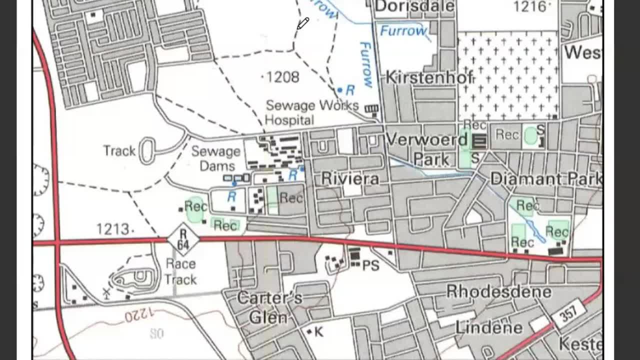 case. so, learners, these are kind of the things that you're looking at, okay. so here is a. i tell your route here. r64, that is cutting through this place. there is a diamond park, there is a cutter's clan- okay, those are just towns. the sewage dams, that means that is a. if you remember about a, 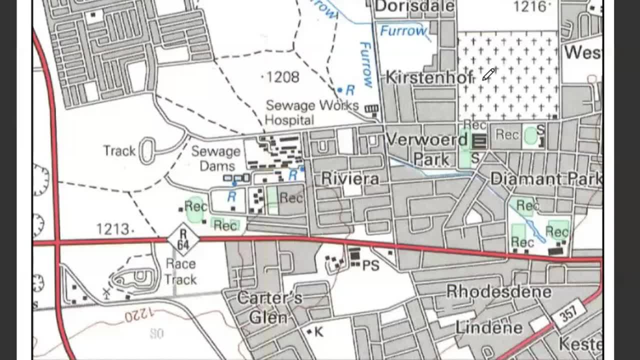 this: if you see sewage and the cemetery in terms of the arrangement of the city, which kind of land use is bad? okay, which kind of values? you can see the park there. there is a park. there is a what, a what, how, a cemetery. there is a sewage. works there somewhere, sewage down somewhere, recreation. 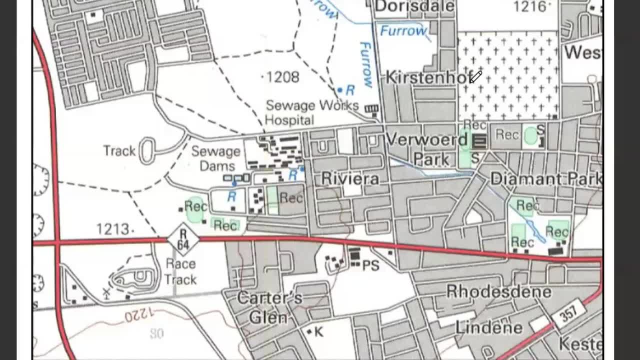 race track, you can see all right. so this is an example, or this is giving you an example, that this one is a transition zone, okay, whereby these activities are basically taking place that way. so you know, sewage- this set is always far right from people because of the smell. 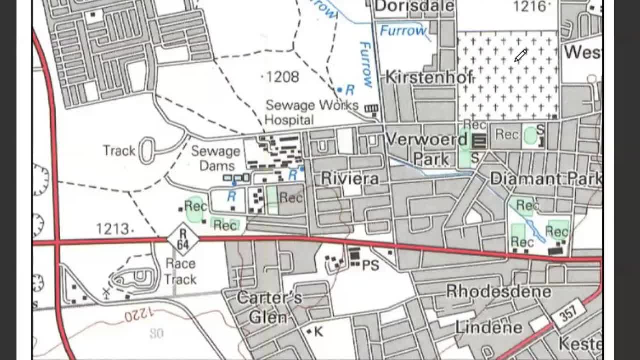 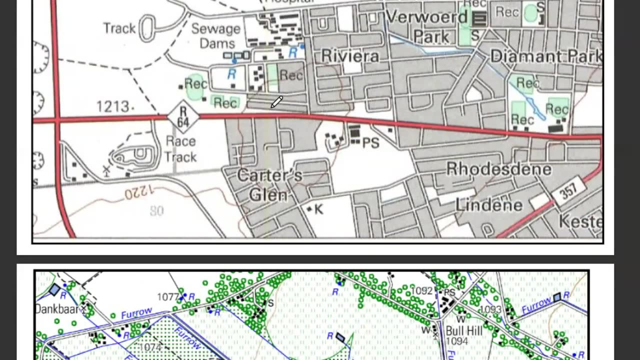 it gives. this one requires very big space, the cemetery, this is a racing track. it also requires a flat area and a bit far away from people. so in this case you get to know that if you are interpreting they can also ask such questions. so if you are interpreting the land use in a certain block, let me say c1 or b1 or c2, remember. 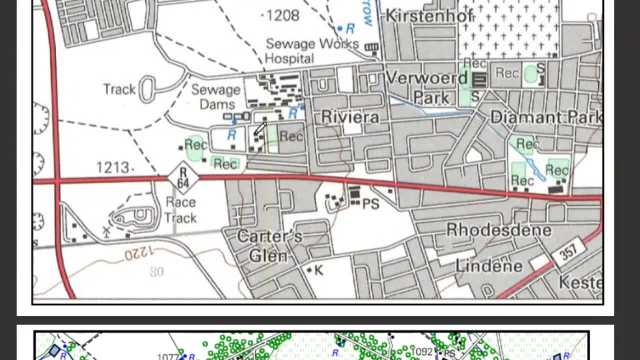 it will be visible on the map. so in this case you look at the possible activities taking place. if it's a central place or if a cbd, which is, it must be lying in the center. so if it's a cbd, it must be lying in the center one. if it's a cbd, it must be connected by other routes towards that. 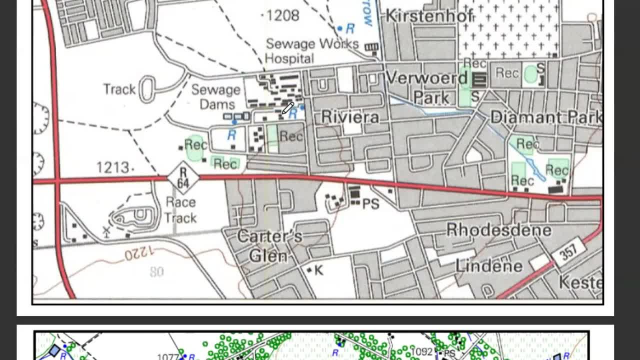 central place that is connecting to it. okay, then the developments that are going to be taking place around it. then we have a transition zone. we have rural urban fringy. okay, the rural urban fringy. we have the rural areas- actually, this one should be right up and fringing. okay, it will run, but not the transition zone- sorry- around urban. 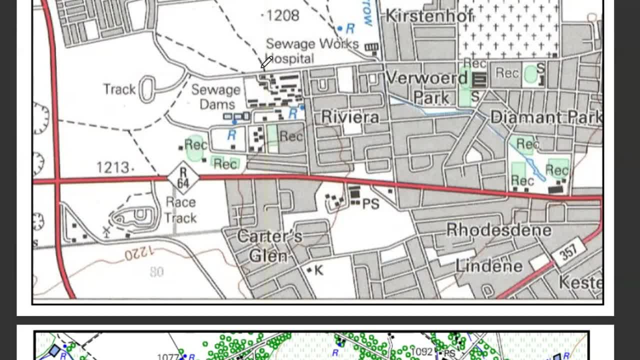 friendly, because a transition zone is the area that has got mixed functions. some some houses appear to be over township area or a township collector. some other houses are tall, some other houses are short, so mixed function is taking place there and no transition zone will have a lot of. 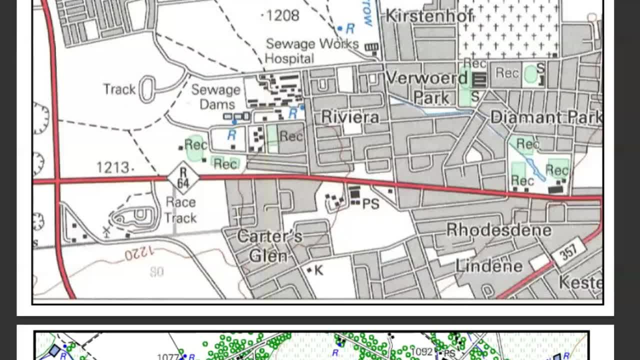 that kind of art there shedding on the walls and all that and so on. so in this case, sorry for that- this area here, the land use around this town, here it should be a rural, urban fringing. so, learners, i want you to note that when they talk about urban fringe, but 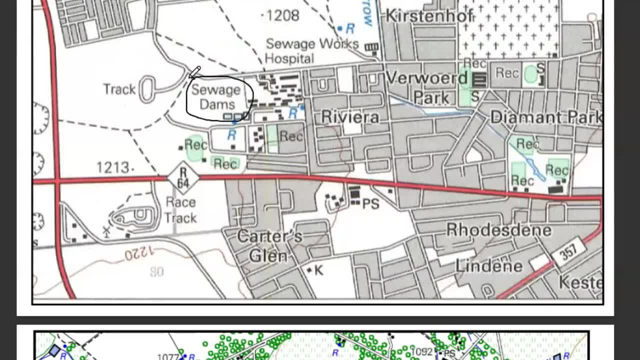 please remember, you must know that the area should have at least any of these activities. number one: sewage terms, sewage works, a cemetery, a golf course, a landing site, a track, a race track, all those kind of activities are taking place in the area that we call a rural, urban fringing. okay. 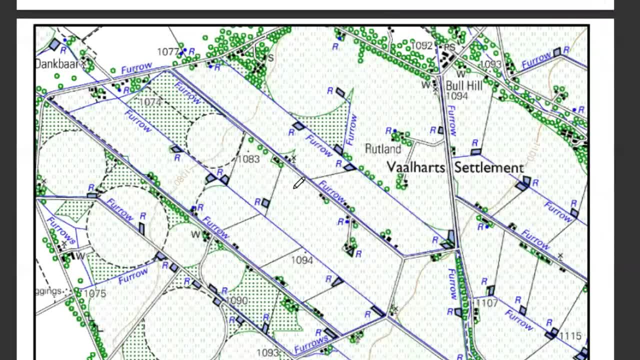 now, which is the dominant activity taking place here, if you look at it? if you look at it, what do you think should be the dominant activity? okay, there are a lot of reservoirs. there are a lot of flowers. okay, which is basically transporting water. row of trees: you can see the row of trees that are built around the water areas. what does? 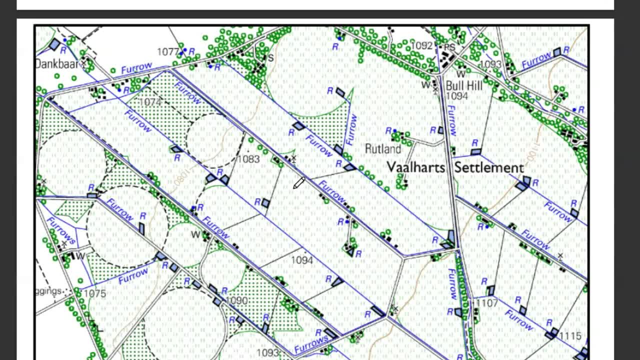 that mean and what does it imply? you know trees provide sheds to the crops. that's number one. okay, trees helps to shield the crops from the very strong winds that are likely to affect the crops on the ground on the farm. so if you see the rock tree, think of the advantages. if it's around the crops, what could? 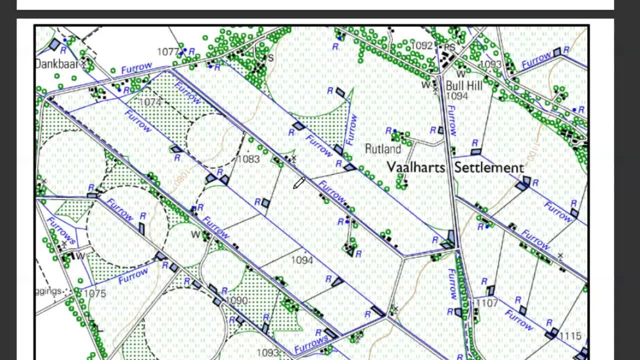 be the advantages. okay, and now when you check this area you can see a bit flatter. that means it can easily favor agriculture, and the flat area also favors easy flow of the drainage systems, the rivers and the water when they want to irrigate this area around here or the crops around the way. 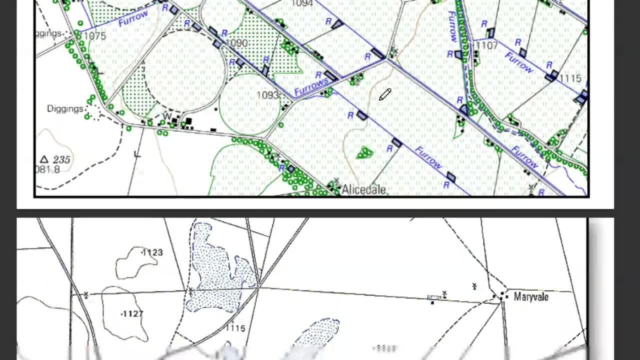 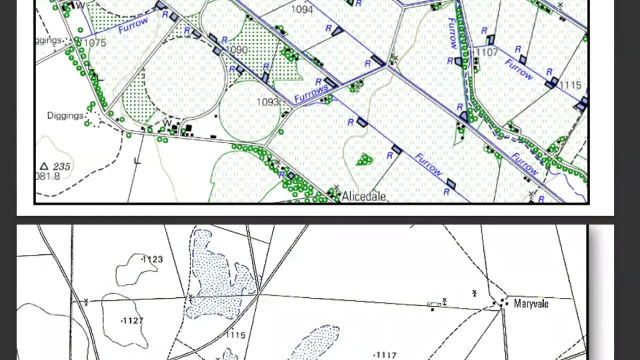 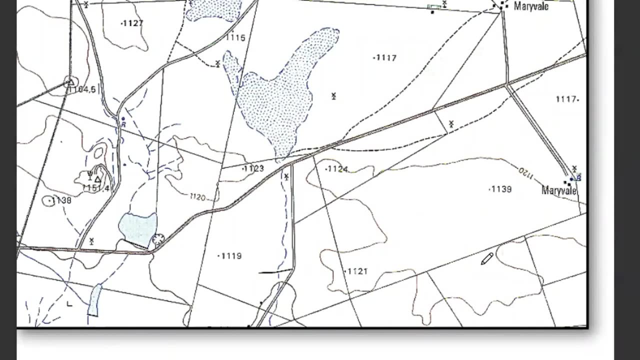 okay, there are a lot of reservoirs, a lot of barrels. so when you look at this area, you can see that this is dominantly an agricultural settlement where agriculture is mainly being practiced. okay, now you check another area. here it's a bit flatter, so it's a low-lying area. 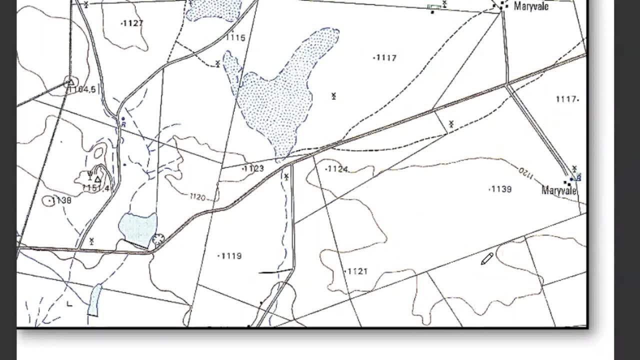 what do you expect? a lot of roads that are connected there, okay, and then a lot of, uh, what you call um seasonal rivers. you look at this. maybe i also forgot to mention that while looking at interpretation, when you talk about, uh, seasonal rivers, it must be a blue line, but broken line, broken dotted line. so it's going. 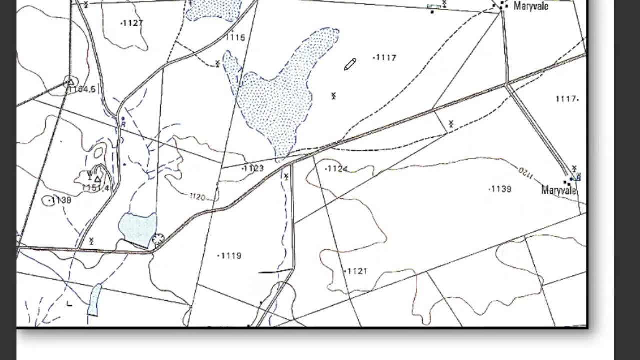 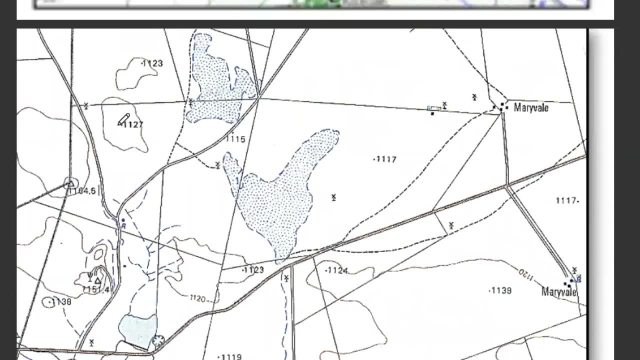 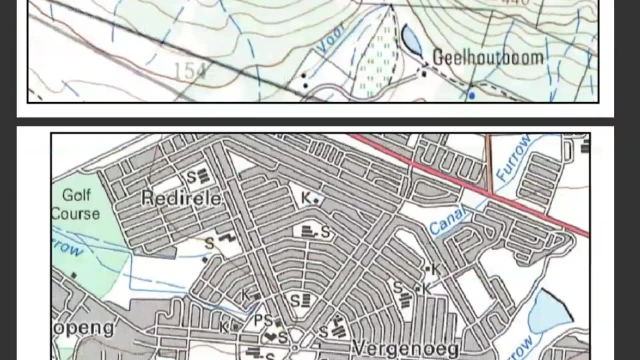 to be seasonal or non-preneur river, okay, or periodic river. so if you see it broken or dotted line, just know it's non-preneur river. if you see it, let me check. compare it with another one that is maybe: um, you look at this one when you check this river here it's giving us an example of what we call. 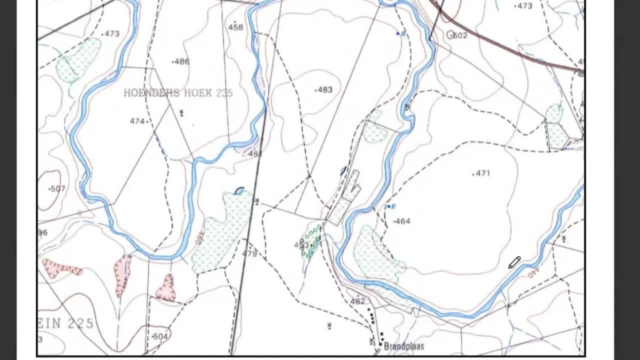 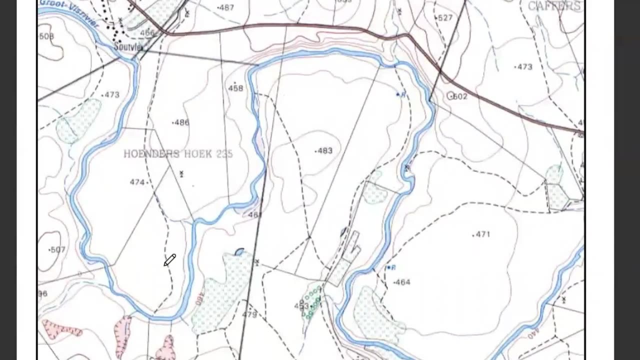 a permanent river. what are permanent rivers? those are rivers that are flowing throughout the year, where the riverbed is always under the water table, both during the dry season and the wet season, so meaning that relationship between the water table and the riverbed uh, is always the water table is. 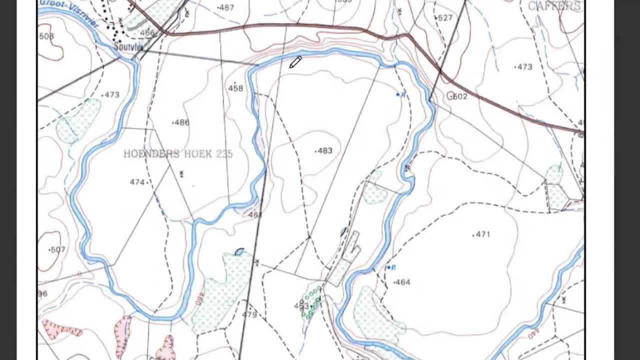 always above the water table. so this river will be flowing throughout the year. so that river, how do you identify it on the map? identify it on the map, if you see it, uh, with the blue line that is continuously, uh, existing. take an example: if this was blue like that, it's going to indicate what you call. 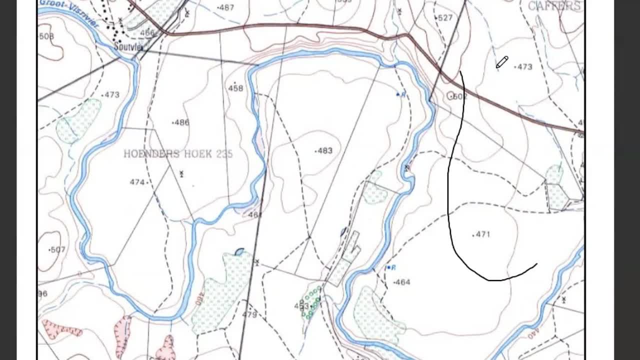 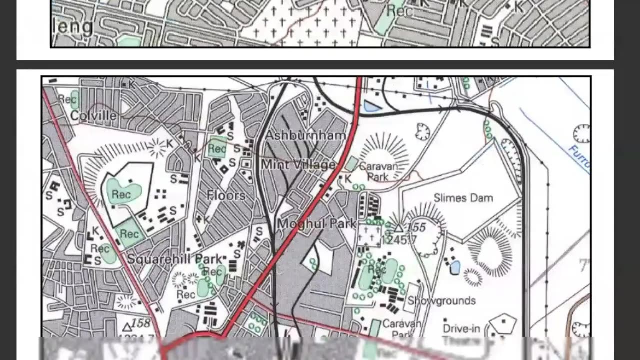 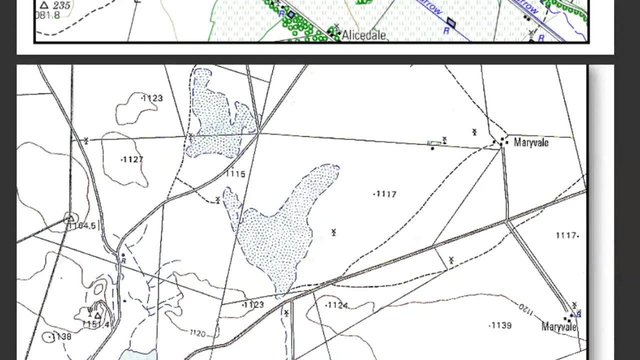 a permanent river, but if it's a broken line like this one, like this one blue but broken line, we call it seasonal river or non-preneur river. so such areas are having such non-preneur rivers. okay. and the last thing that i want us to look at is this part here on the map, um, this part here you can see in terms of its gradient. 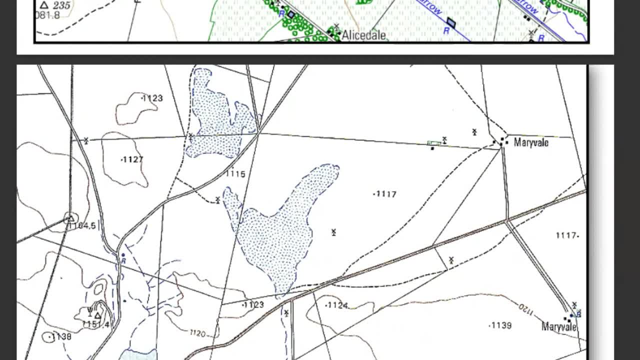 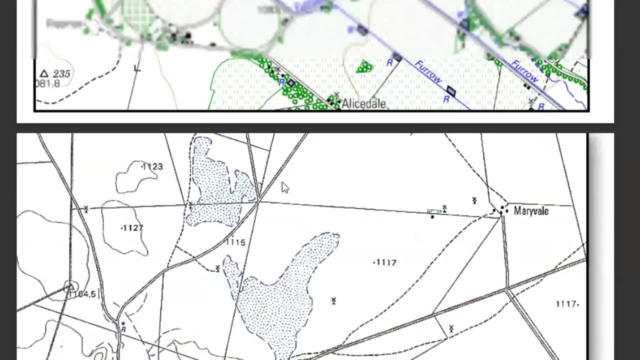 it is a very flat area, depending on the nature of the contour lines. you can easily see them. you can even see the way the water is existing, like there are a lot of several pockets of water that is um colonized within one area and that means that area is a bit flatter. so hope learners i have. 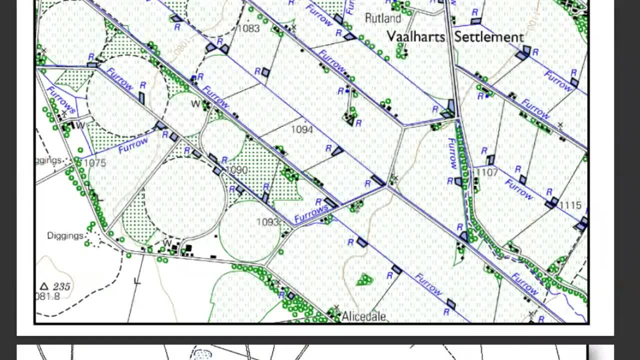 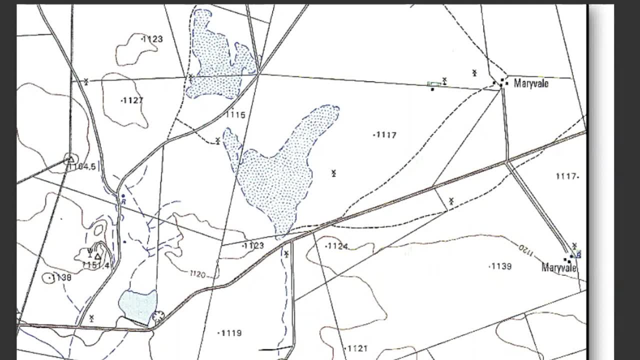 not left out anything related to interpretation. so please get in position to be in position to tell in summary or in a nutshell, been positioned to tell how all the topics you have looked at, both in paper one and paper two, how can they be applied on the map. everything that you look at is 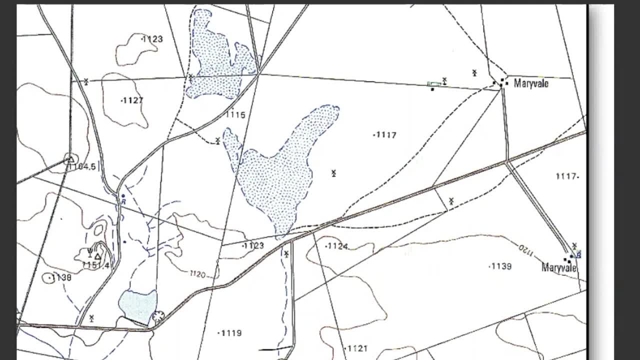 very, very, very important. It's very, very important in order to apply it on the male. If there is anything that I have not interpreted for you, please be in position to leave your comment. be in position to let us know that you really need that aspect.